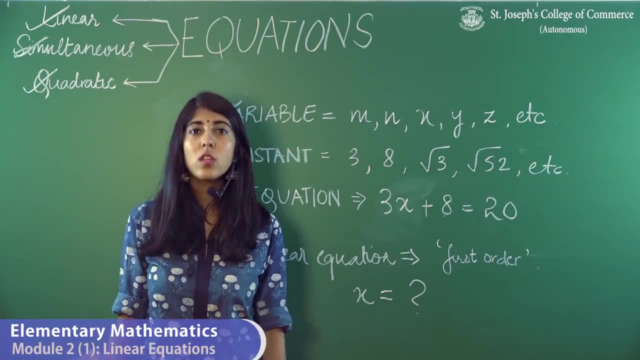 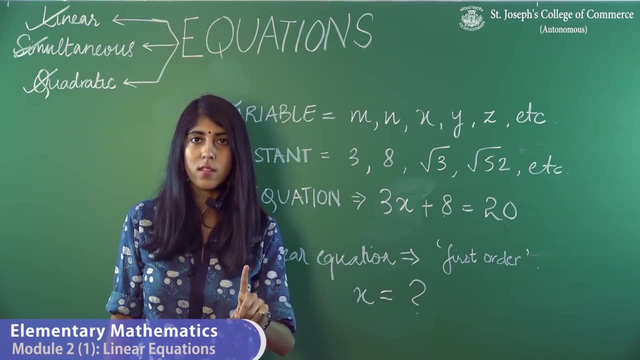 equation is A linear equation is any equation which is in the first order. The first order means that the value or the answer to it has only one answer. So the root of a linear equation or the answer of a linear equation has only one value to it. Now, when 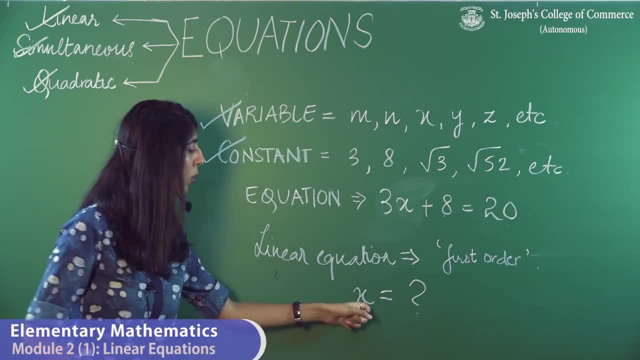 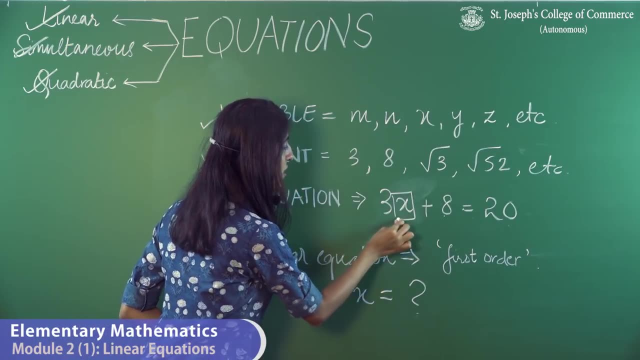 you have to try to find out the value of it. you normally try to find out what the value of x is. That is what you need to do in a linear equation. Now, why it is called in the first order is because the variable, the highest power of the variable, is 1 and cannot. 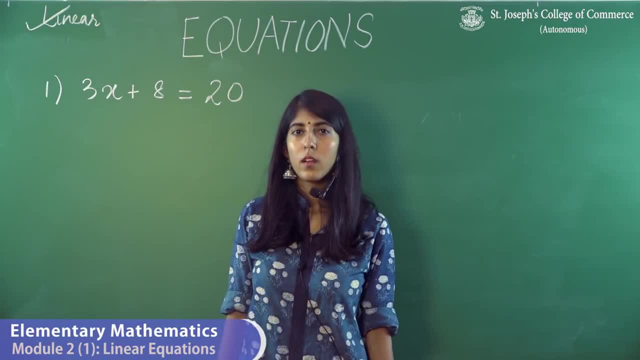 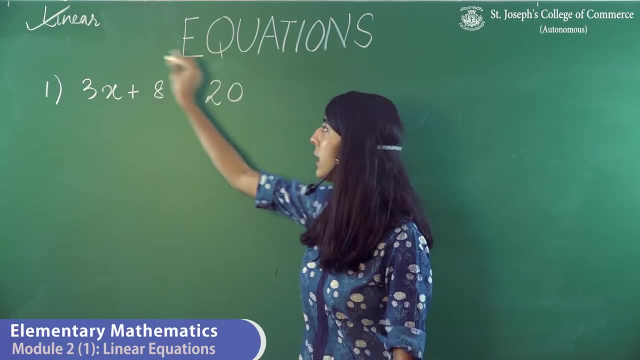 exceed 1.. This is the example of the equation that we took in the previous thing: 3x plus 8 is equal to 20.. In this equation, 3x is the variable part of it and 8 and 20 are the constants. 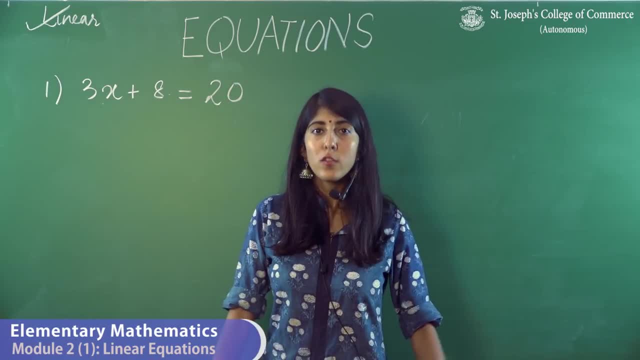 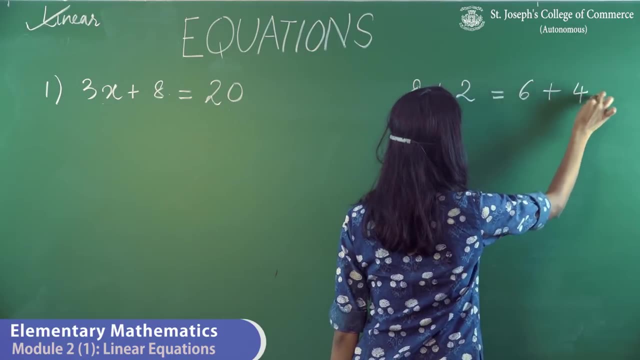 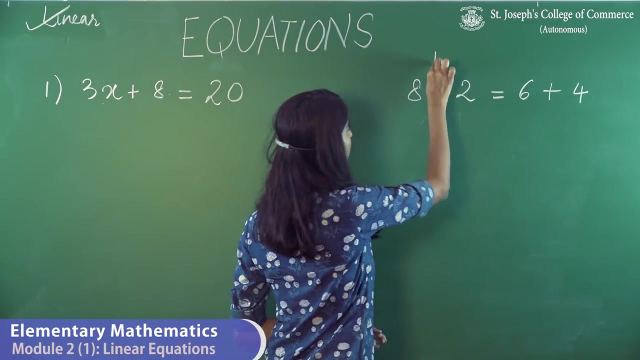 Let's move on to find the origin of solving a linear equation. If we notice, these two sides are bifurcated or separated by an equal to sign. sign. Let's call this the left hand side of the equation and that the right hand side. 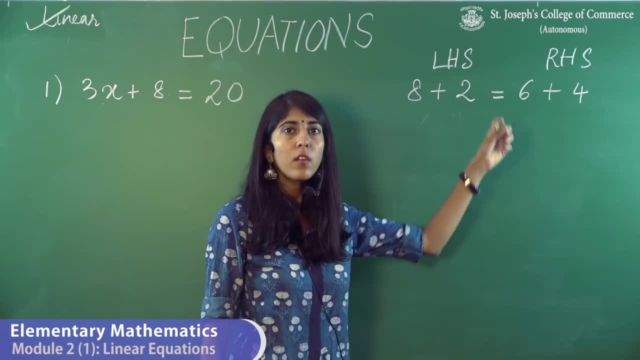 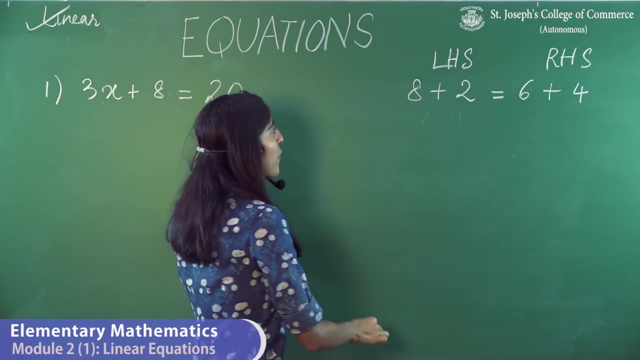 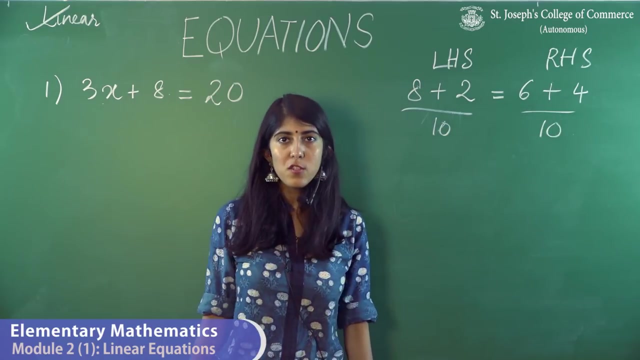 of the equation. If you notice, in an equation the left hand side is always equal to the right hand side and it is separated by an equal to sign. When we have to solve it, we realize that 8 plus 2 is equal to 10 and 6 plus 4 is equal to 10.. The first rule we apply 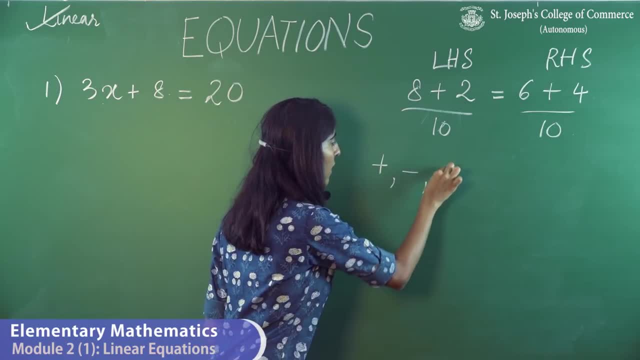 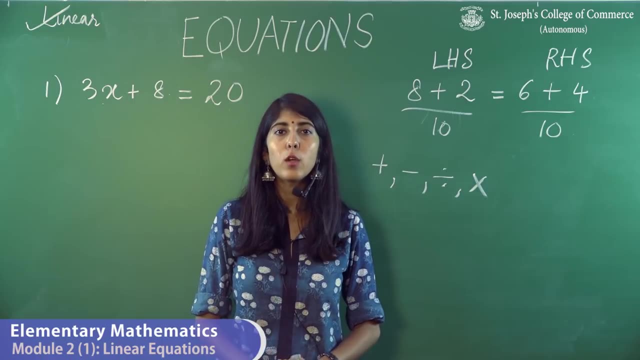 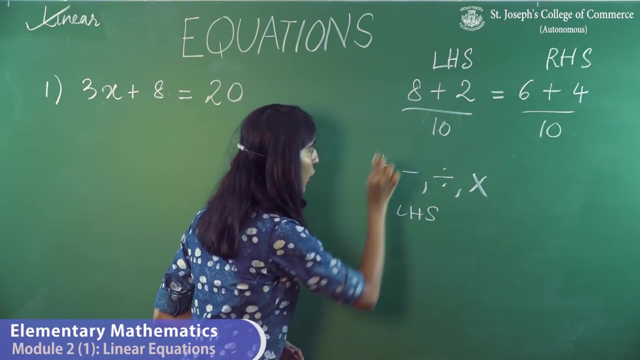 is the fact that if you add, subtract, divide or multiply both sides of the equation with the same variable or constant, the value of it does not alter or change. Let's take, for example, if I take the left hand side and I add a 2 to it, So it's 8 plus 2 plus 2, and 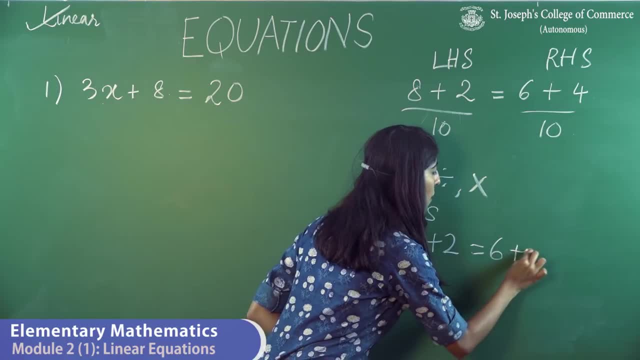 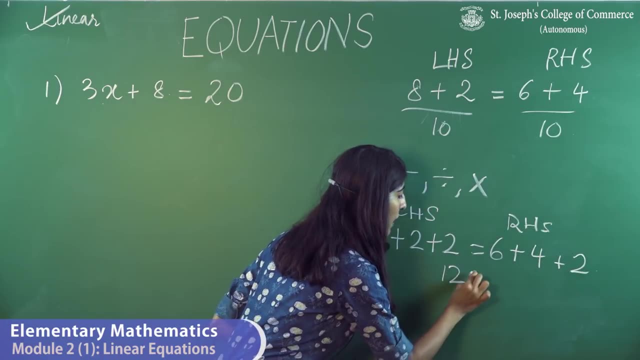 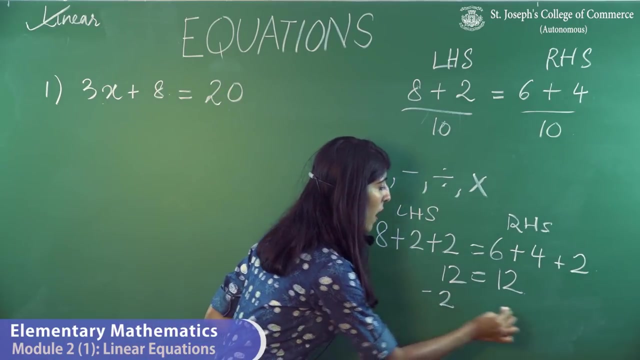 I add the same number on the other side as well, So it's 6 plus 4 plus 2.. The value on both sides of the equation is equal to 10.. Remain 12 and they are equal. This satisfies this rule If I subtract 2 and I subtract. 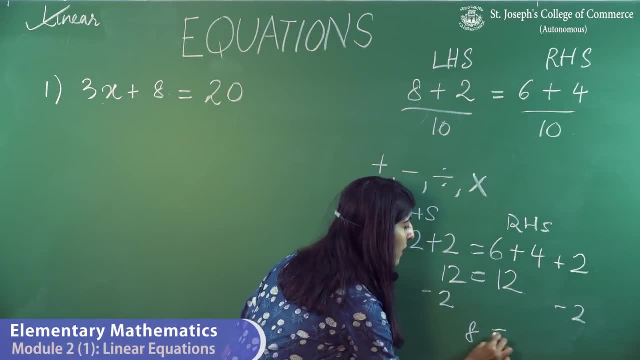 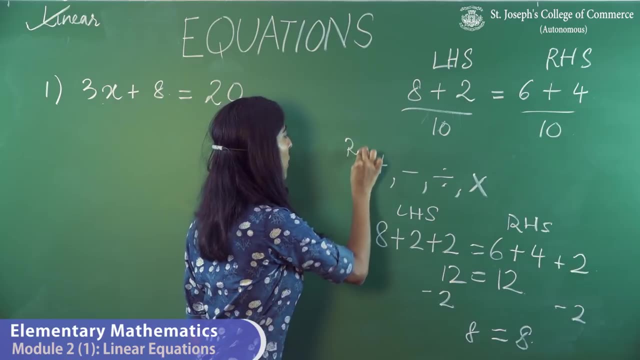 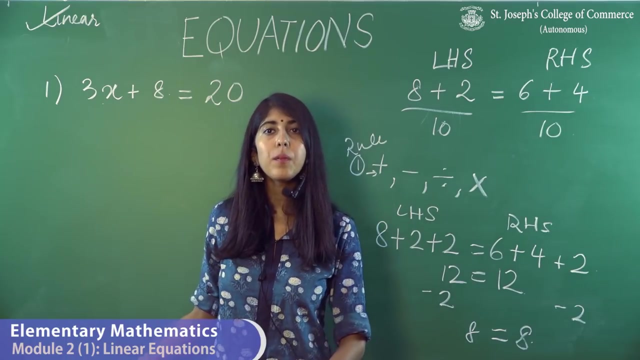 2 from both sides of the equation, the value of it will be the same as it is 8.. Although the value of it changes, both the values are equal. That is what rule number 1 states. This is the origin of solving a linear equation. When you look at it practically, we solve it. 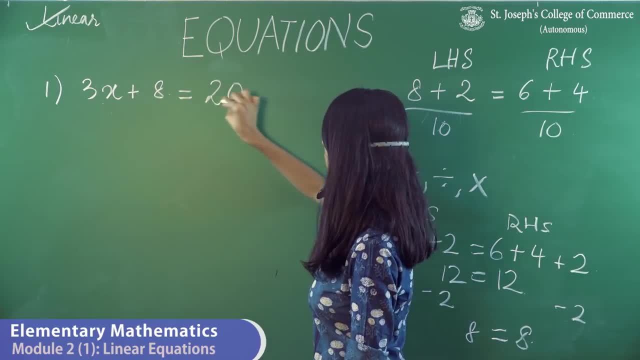 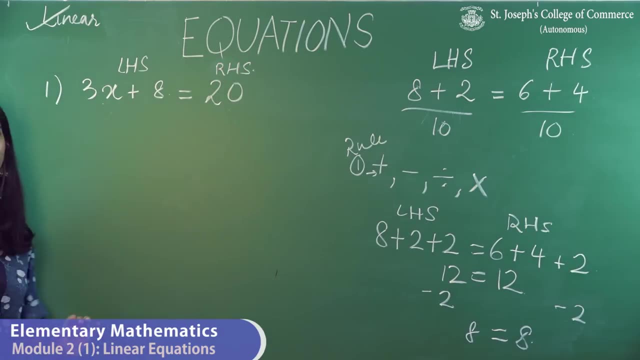 in an easier way. When you look at, 3x plus 8 is equal to 20. as I said, this is the left hand side and this is the right hand side. What we do is we transfer all the constants to this side and all the 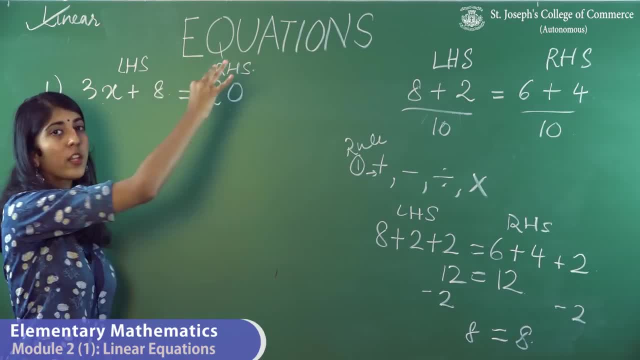 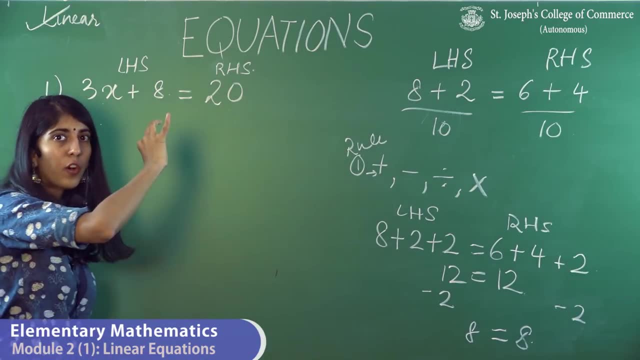 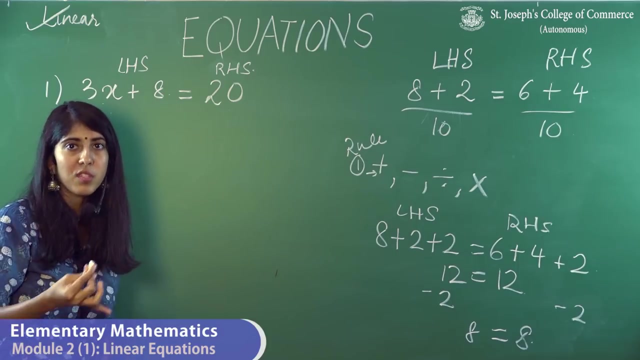 variables onto one side. So let's do all the constants on the right hand side and all the variables on the left hand side. So one more thing we need to remember is when we transfer any variable or constant from one side to the other, The sign of it changes and becomes the opposite, For example, the sign preceding the variable. 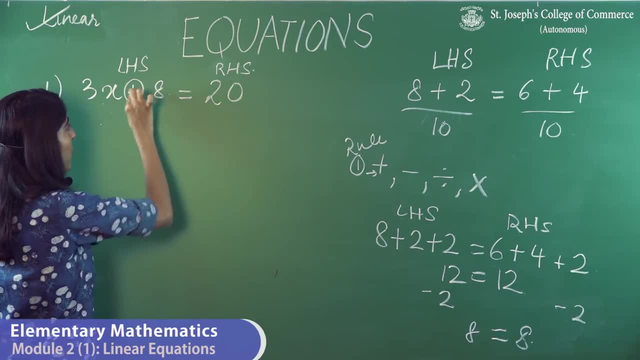 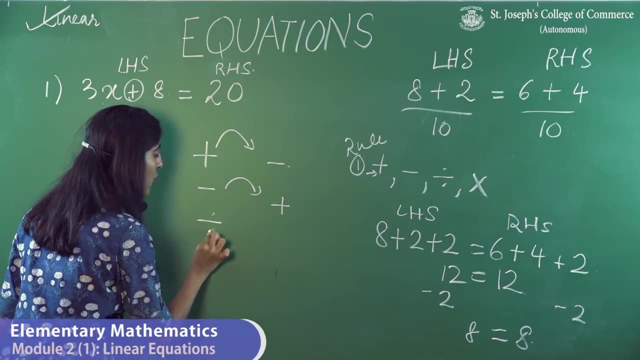 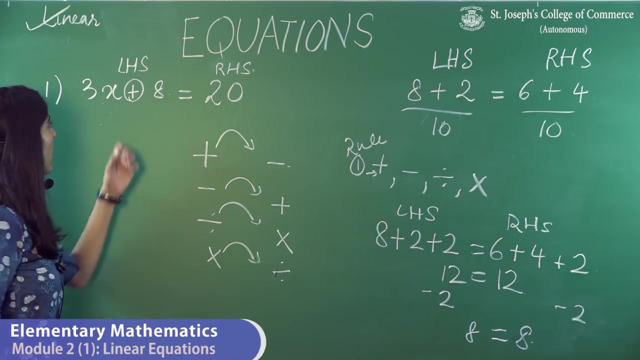 or constant will become opposite. Let's see over here it's plus. So the rules that you need to remember is: plus becomes minus, minus becomes plus, division becomes multiplication and multiplication becomes division. When we are solving it, since we are transferring all the constants to the right hand side, what we are going to do is 8 should be transferred. 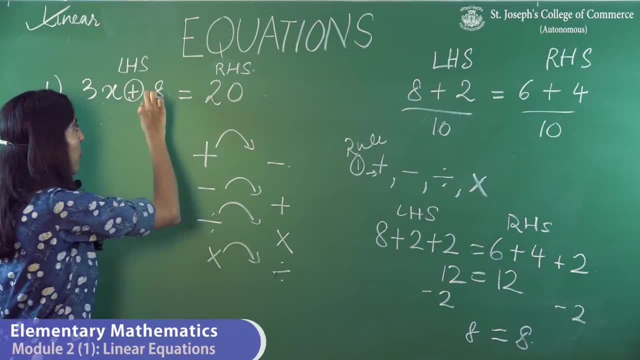 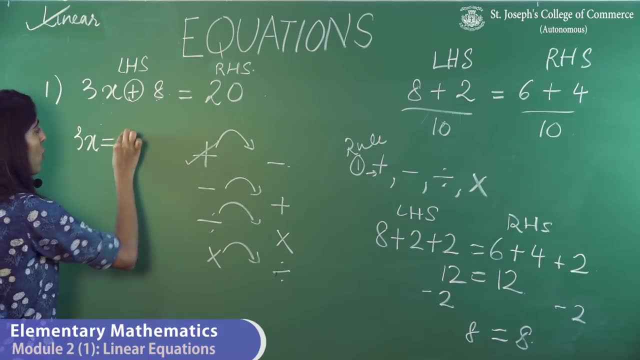 to the right hand side, 8 is preceded by a plus sign. The plus, when it is shifted to the other side, will become minus. So we are applying this rule. So 3x is equal to 20, plus will go here and it will become minus 8.. When we solve it, 3x is equal to 20, minus 8 is equal. 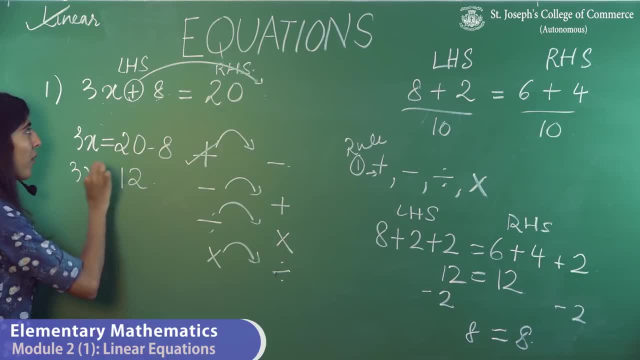 to 12.. The next step is to find the value of x. The concept of a linear equation is to find the value of x. In a linear equation, x has only one value. So when you are solving it, you realise that 3 is multiplied to x and is equal to 12.. When 3 is separated from the x, it is now a constant. 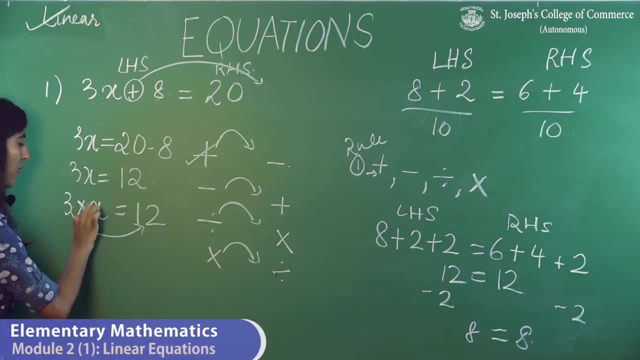 So when it is transferred to the other side, it is multiplied to x and hence, when it is transferred to the right hand side, it becomes division. So you apply this rule. So 3 into x is equal to 12.. x is equal to 12 divided by 3.. 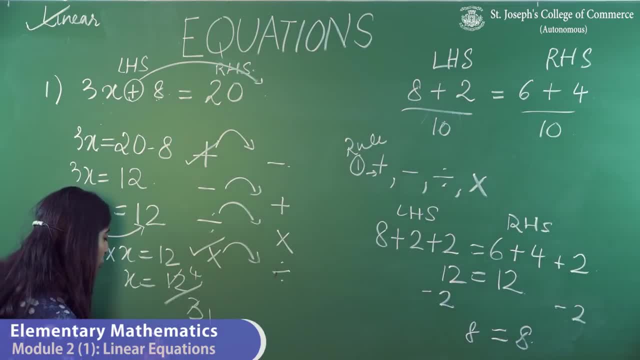 When you solve it, 3x is equal to 12.. x is equal to 12 divided by 3.. When you solve it, 3 ones are 3, fours are. Therefore, the value of x is equal to 4.. As you can see, it is a. 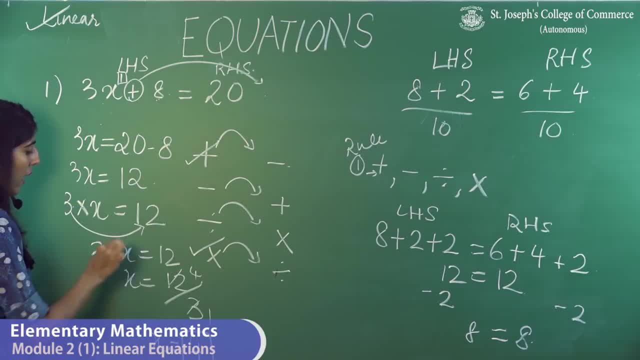 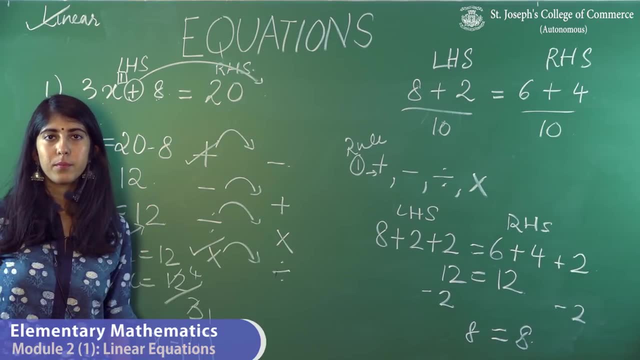 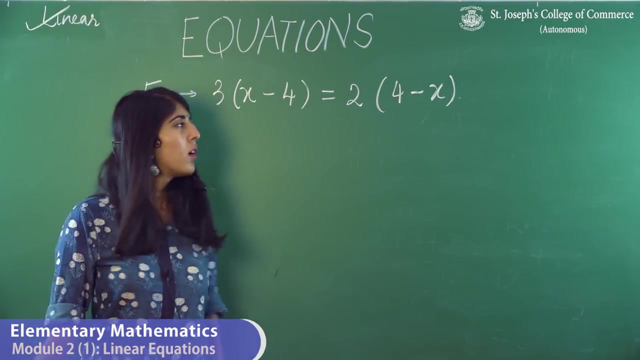 linear equation and the highest power of x is equal to 1 and therefore the root of it has only one answer, and hence x is equal to 4.. We are going to try solving another example. So 3 into x minus 4 is equal to 2 into 4 minus. 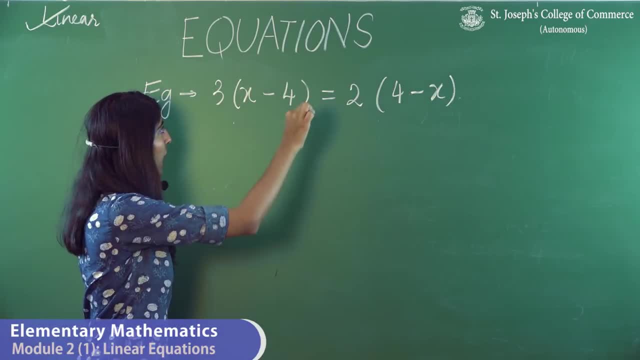 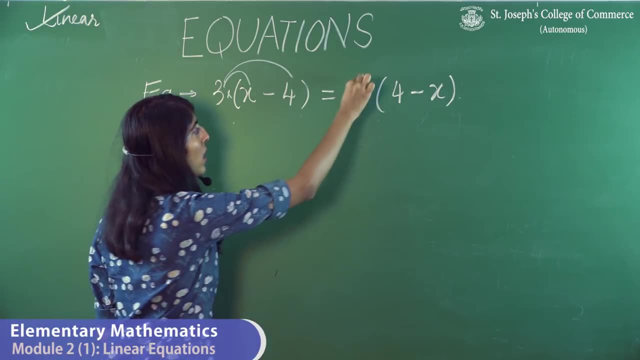 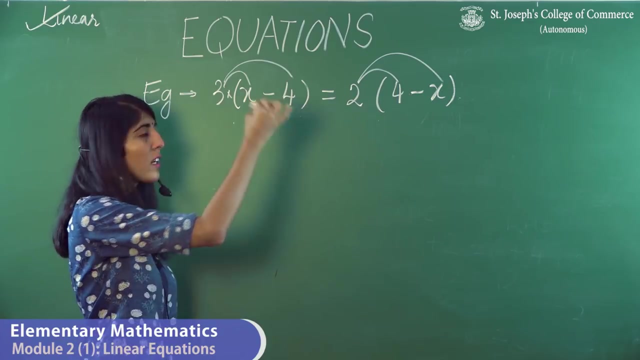 x. When you are solving any sum with a bracket, this means that the 3 is multiplied with the x and it is multiplied with the minus 4.. Same way, 2 is multiplied with the 4 and it is multiplied with the minus x. Before we look into the segregation of left hand side and right hand, 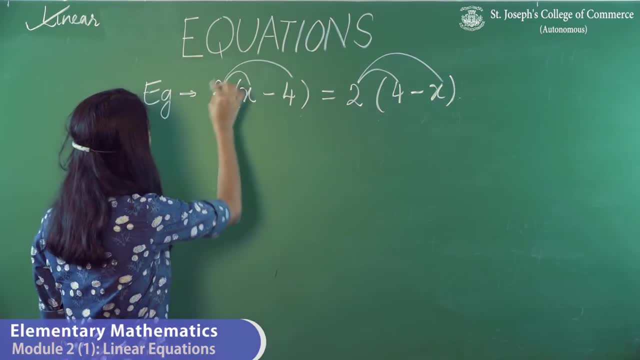 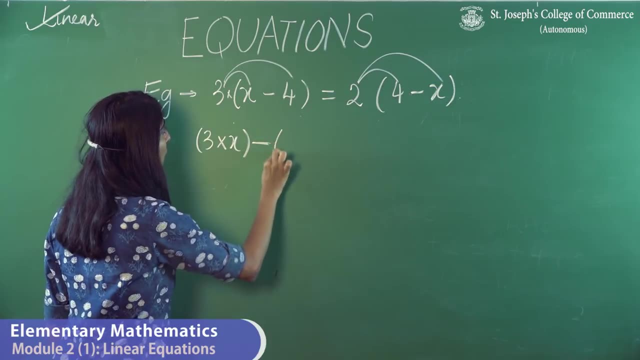 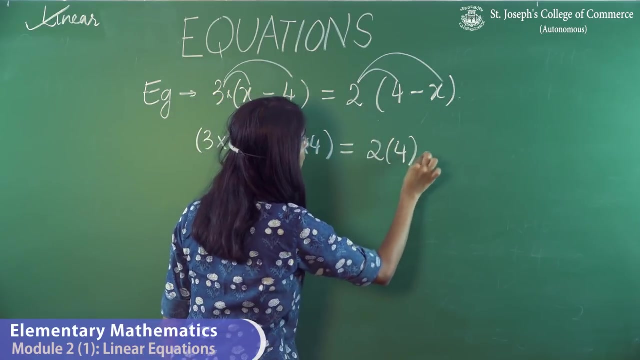 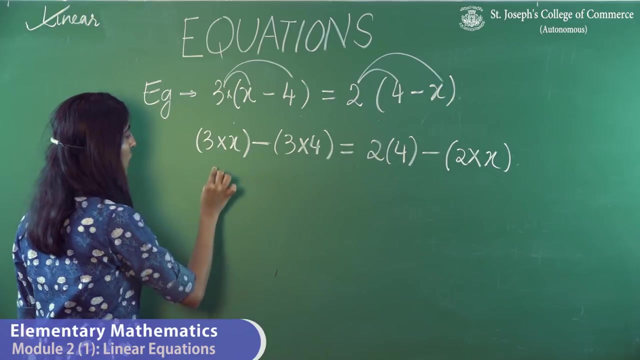 side. let's just expand the brackets using Bodma's rule. Now, when you expand it, 3 into x, So this becomes 3 into x minus- remember the minus sign, and this will be 3 into x, 3 into 4.. It is equal to 2 into 4 minus 2 into x. As we solve it, 3 into x is 3x minus. 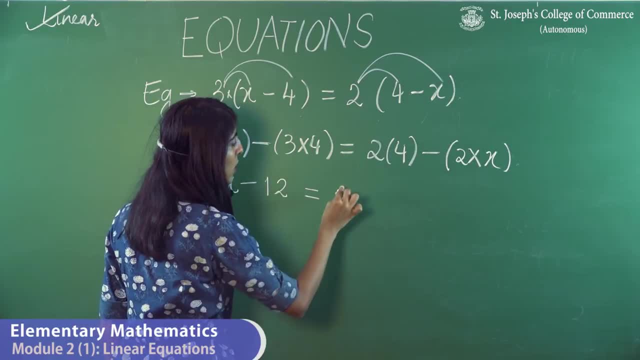 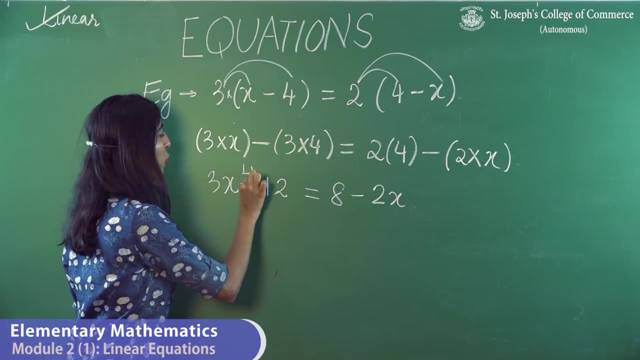 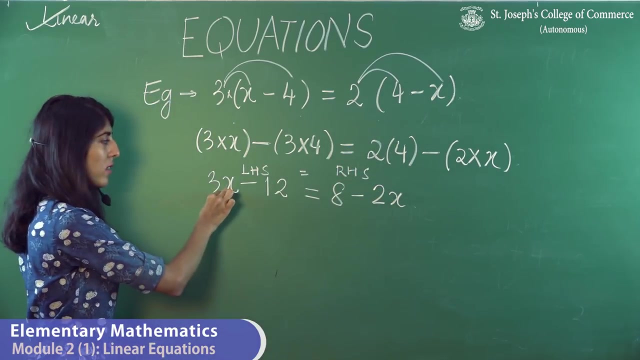 3 into 4 is minus 12 is equal to 2 into 4 is 8, and 2 into x is 2x. Now we apply the rule that I taught you before: LHS is equal to RHS. Now we transfer all the variables to this side and all the constants to the right hand. 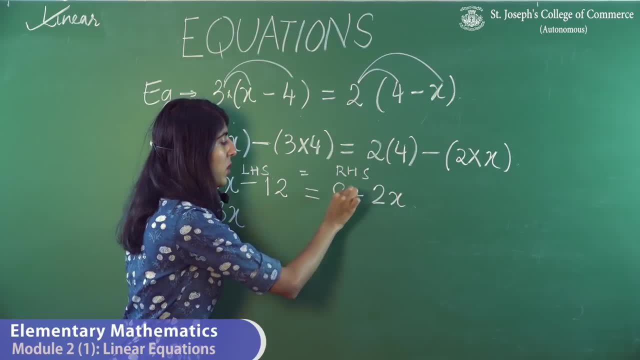 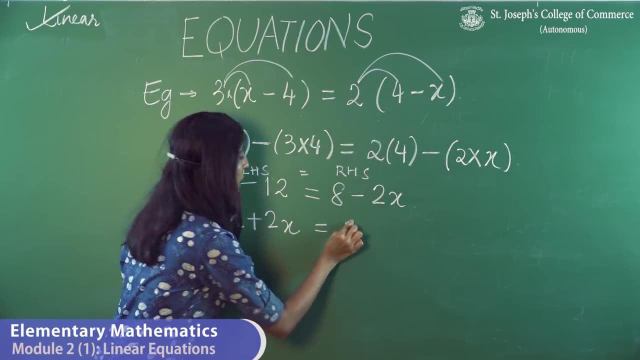 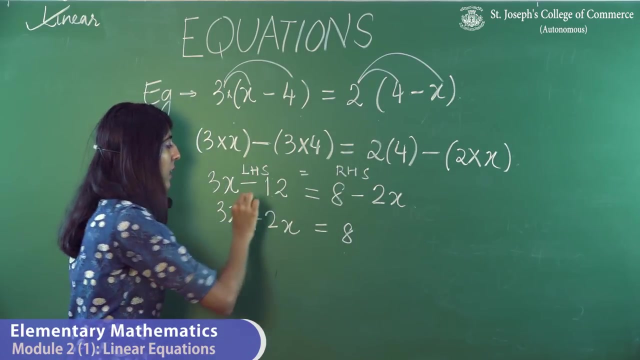 side. When we transfer the variable 2x is preceded by a minus sign. So when it is shifted to the other side, it becomes plus 2x. 8 remains as it is, since we are transferring all the constants to this side. When we transfer 12 to the other side, it is preceded by a negative. 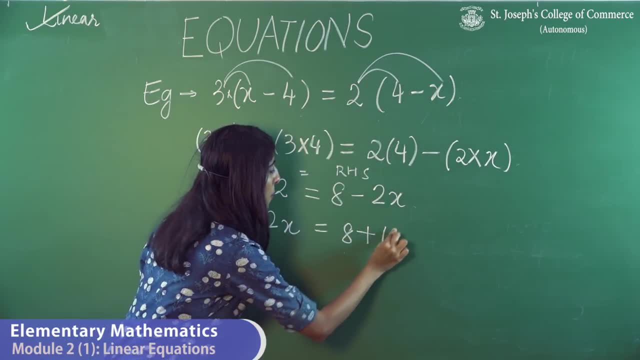 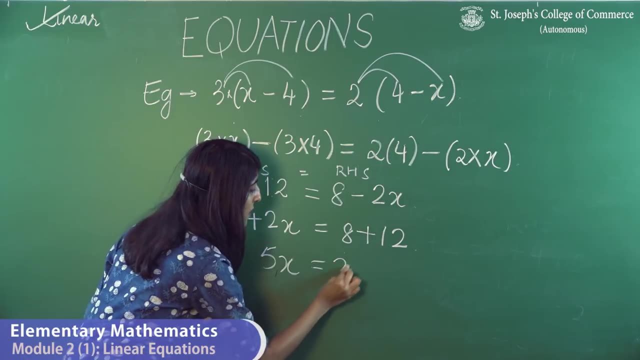 sign. So when minus goes to the other side, it becomes plus 12.. So 3x plus 2x is equal to 5x, and 8 plus 12 is equal to 20.. As I said, 5x is actually 5. 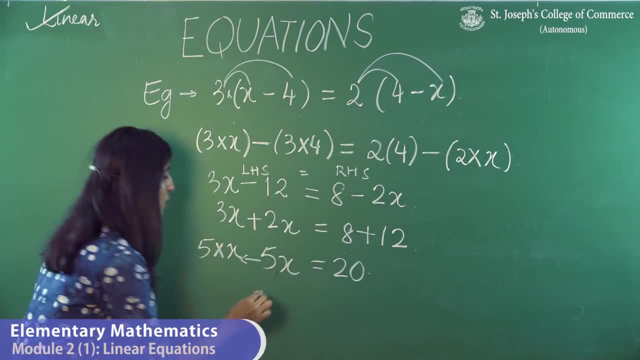 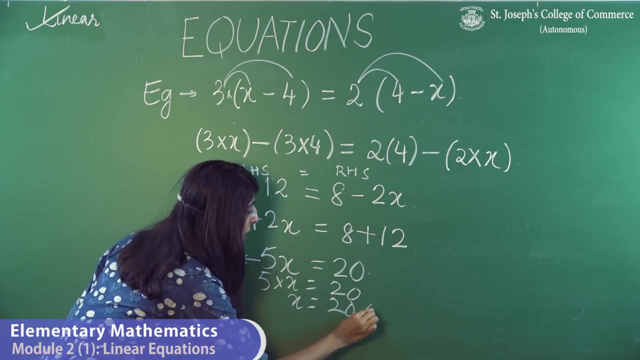 into x. So when you do 5 into x is equal to 20.. x is equal to 20 divided by 5, because multiplication, when it goes to the other side, will become division. So 20 by 5, therefore, the value of x is equal to 20.. 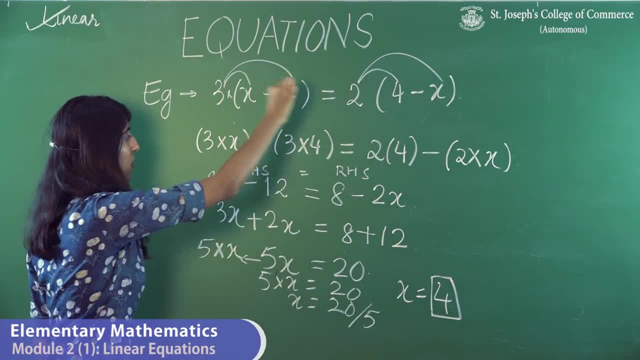 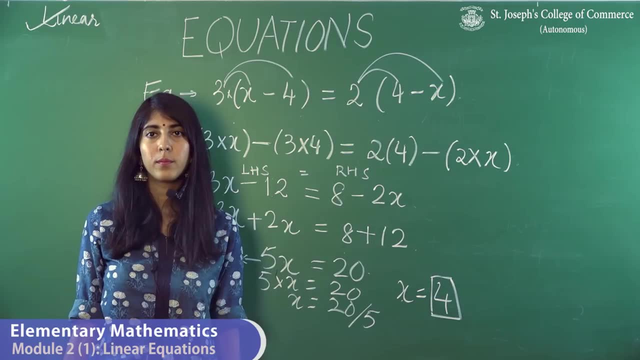 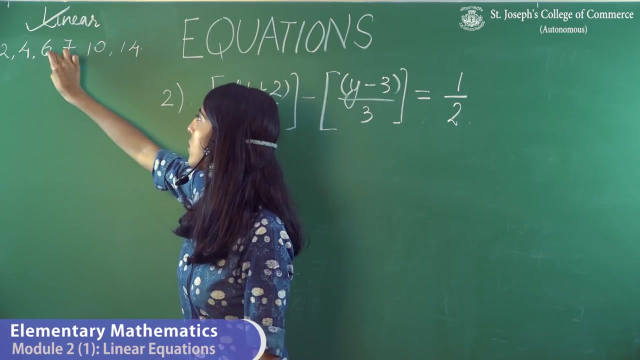 4. Linear equation. There is only one variable throughout, So the variable has only one answer to it. So therefore, x is equal to 4.. We are going to be solving the second, fourth, sixth, seventh, tenth and fourteenth sum under: 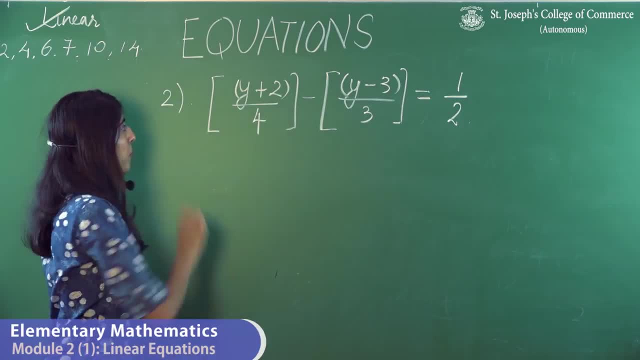 linear equations in the handout. Let's start with the second sum: y plus 2 divided by 4, minus y minus 3 divided by 3 is equal to half, So reference this as y plus 3 divided by 5.. We are going to be solving the second, fourth, sixth and tenth sums, So this is going to 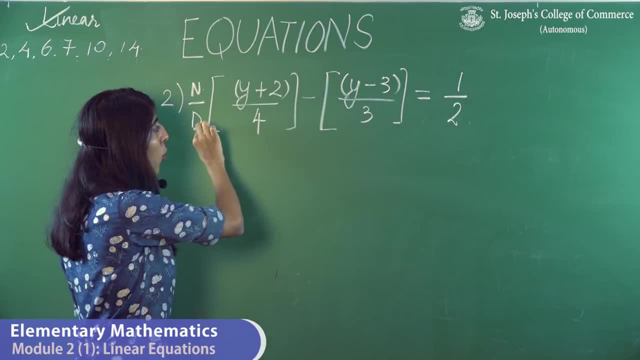 be like a 2 and in the third one. So what we want to do is find a denominator and a denominator And if you notice, there is a numerator and a denominator involved in this question. When a numerator and a denominator gets into the picture, you need to start by finding the LCM of the denominators. Let's 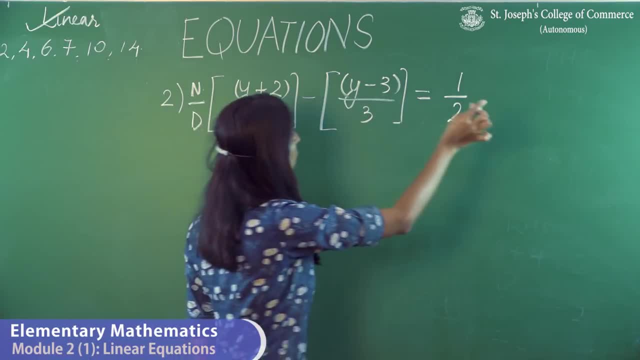 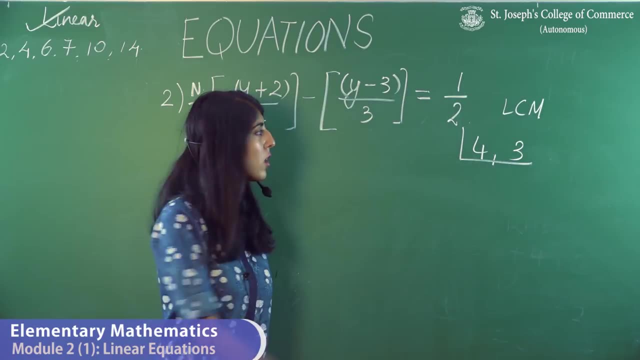 start with the left hand side, as it has more number of values. Now, when you find the LCM of 4 and 3, we have covered this under module 1.. So LCM of 4 and 3 starts with the least number, 2.. 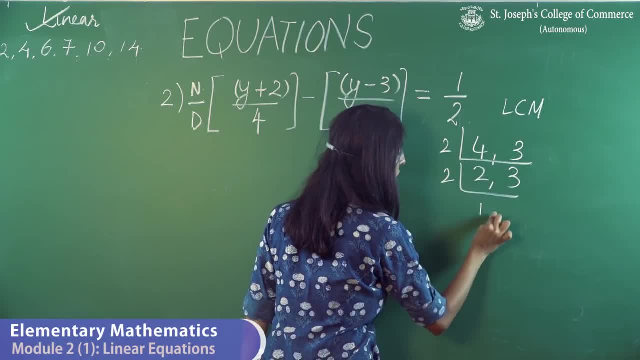 So 2 and 3 start with 2 again plus 1.. So then we have the second number and the number 3.. Okay, Let's go back to our first one, And here we have the destination. So we have the left. 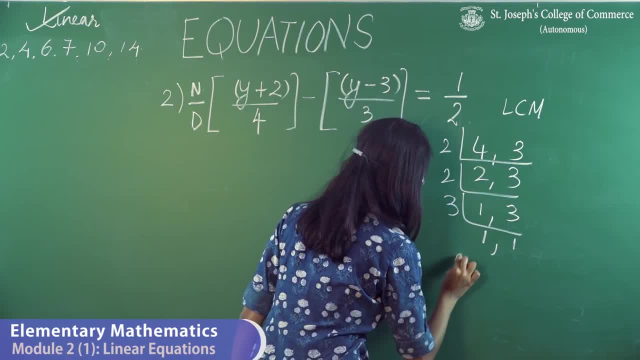 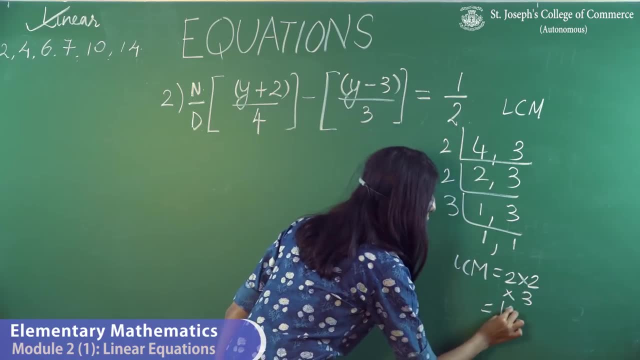 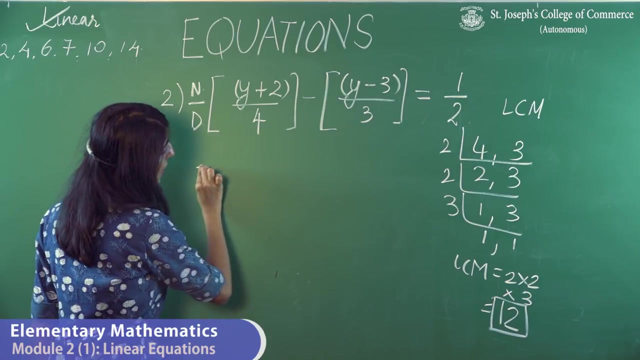 1 and 3, 1 and 1.. LCM will be 2 into 2 into 3.. So therefore the LCM of the denominator of this left-hand side of it is 12.. So the second step is by directly writing a denominator as 12.. 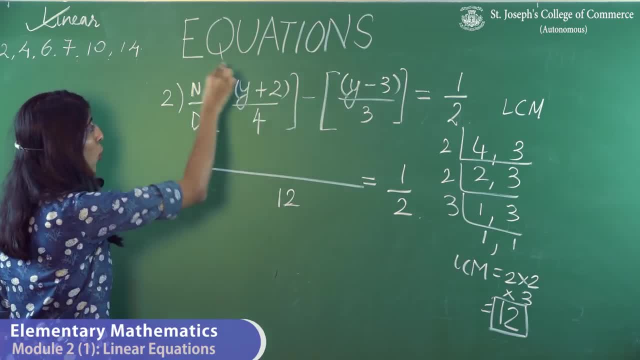 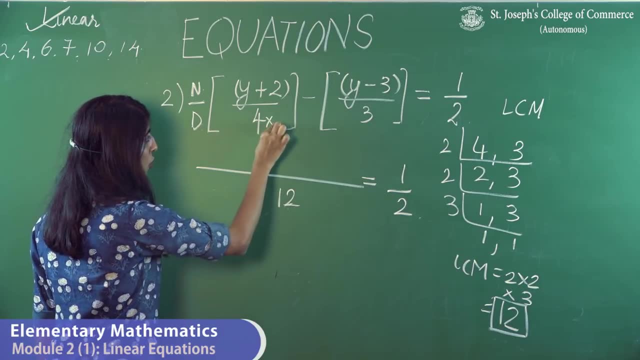 So when we write the denominator as 12, we need to coordinate with the numerator. So if this is 4,, 4 into what number gives you 12? 3.. So you need to multiply the denominator by 3 and the numerator by 3.. 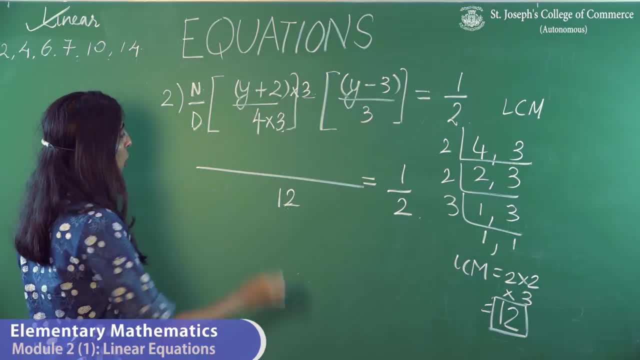 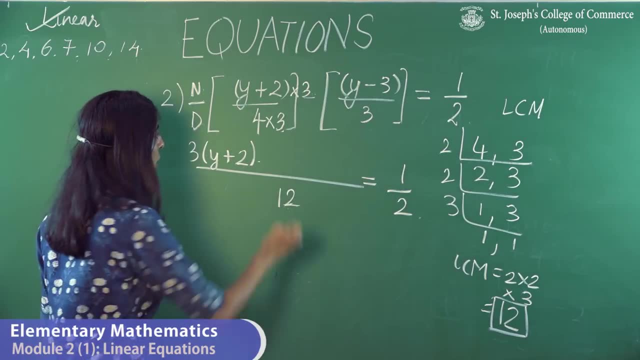 That is the rule when you're trying to solve using LCM. When you multiply the numerator by 3, it becomes 3 into y plus 2.. Do not forget the minus sign. Let's leave it as it is: 3 and 12.. 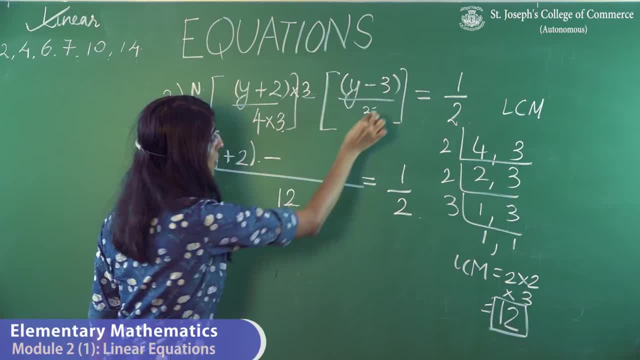 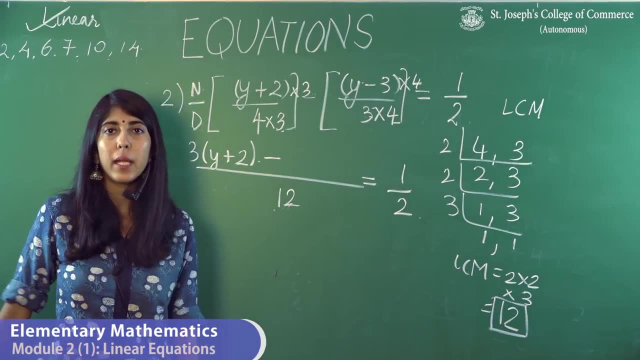 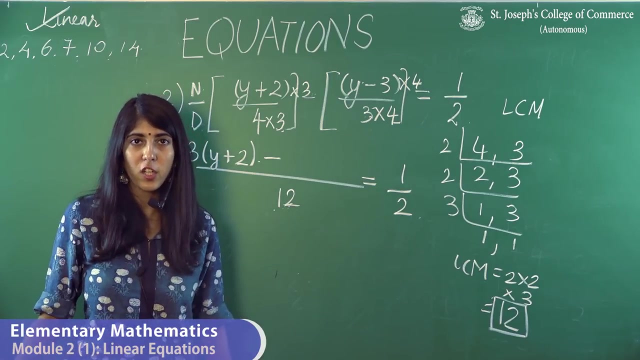 When you check the following: 3 into what gives you 12?? 3 into 4 gives you 12.. That means that the numerator and the denominator should both be multiplied by 4.. The reason you do this is so that the value of the denominator and the numerator as a fraction does not change. 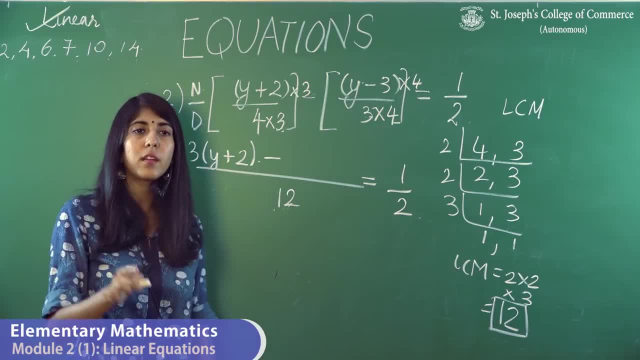 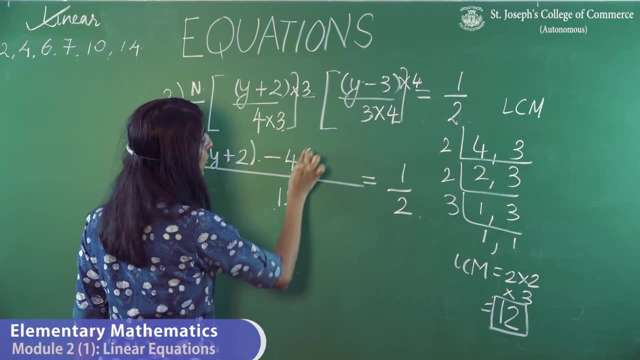 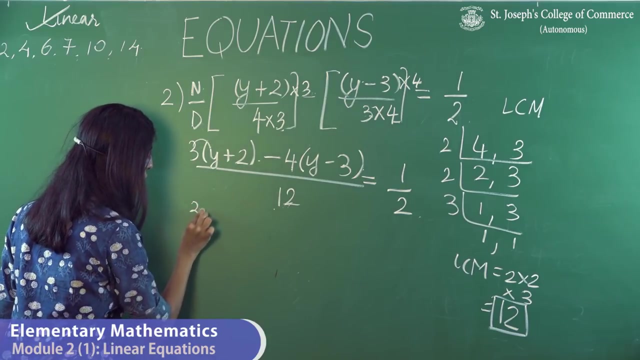 Which is why you're multiplying and dividing both the numerator and denominator by the same variable or constant. When you multiply the numerator by 4, you write 4 here and y minus 3 inside the brackets. As you solve it, 3 into y gives you 3y. 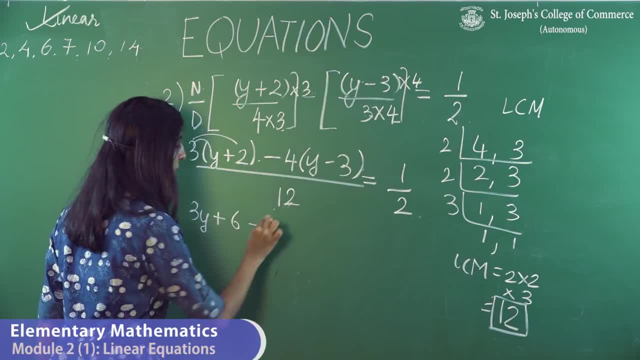 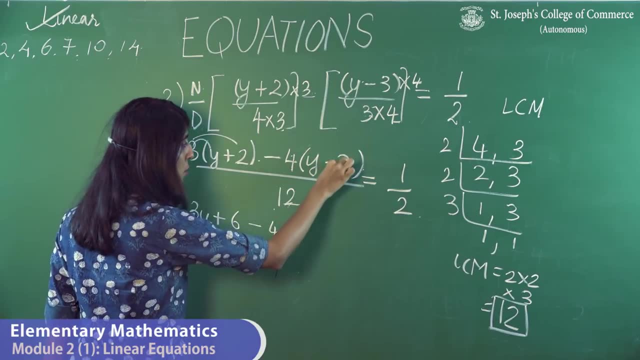 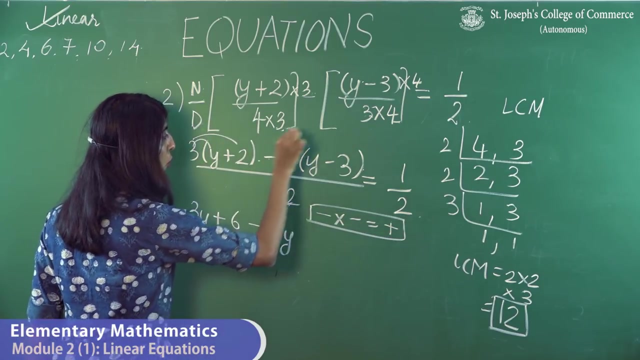 3 into 2 gives you 6.. Minus sign: Do not forget the minus sign. 4 into y gives you 4y And minus 4 into minus 3.. Remember: minus into minus is equal to plus. So minus 4 into minus 3 will give you plus 12.. 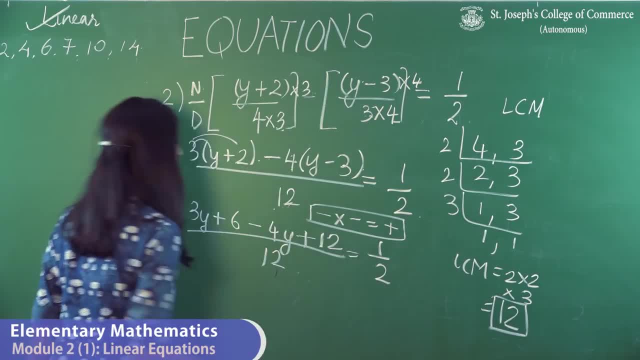 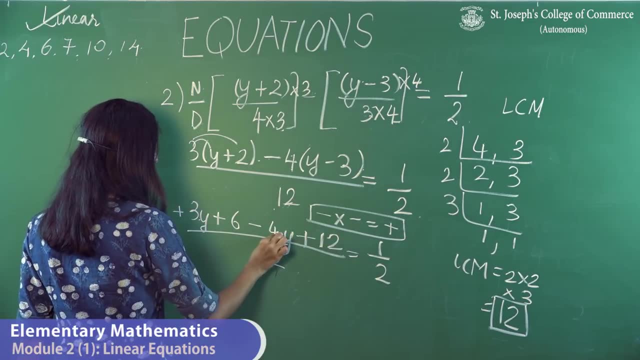 Leave the rest of it as it is is equal to half. Solve the numerator 3y minus 4y, So it's plus 3y minus 4y. That means when the signs are opposite you need to subtract. 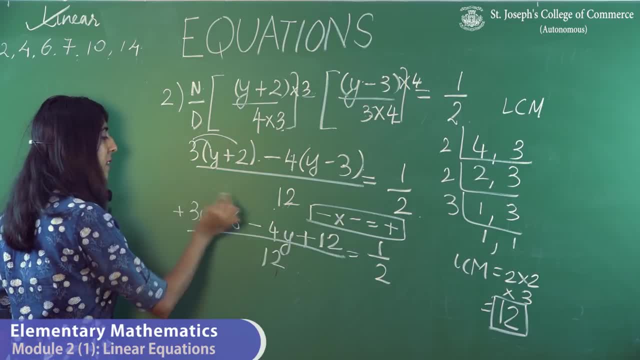 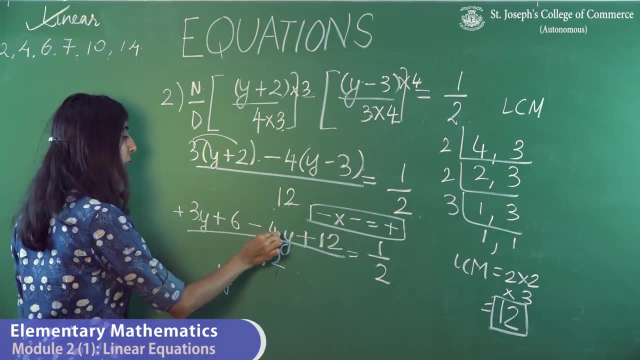 We've done this under the first module, under number line. So when the signs are opposite, you need to subtract: 4 minus 3 is 1y. 4y minus 3y is equal to 1y. The sign preceding a greater value is a negative sign. 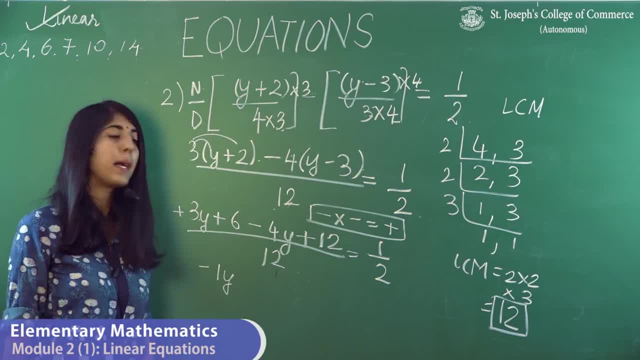 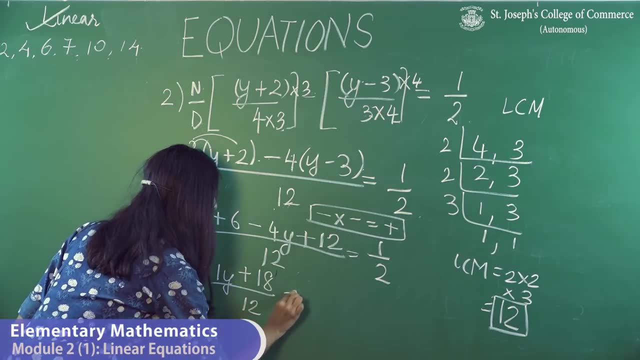 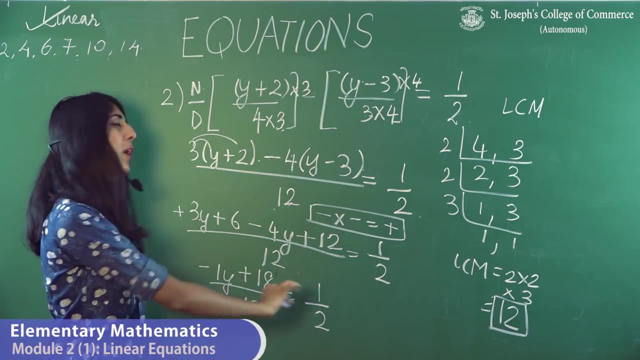 Which is why 1y will be preceded by a minus sign. When you solve the rest. 6 plus 12 will give you 4y. 4 plus 12 will give you 18.. Leave the rest as it is When you have to solve it. when it comes to this, there's no other way you can simplify it except to cross multiply. 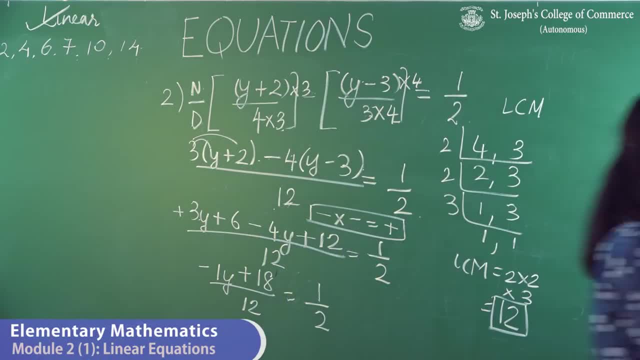 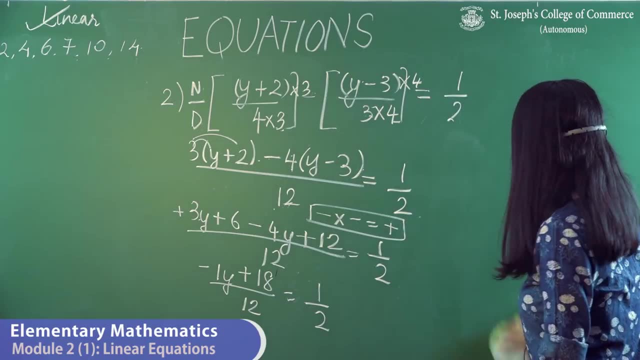 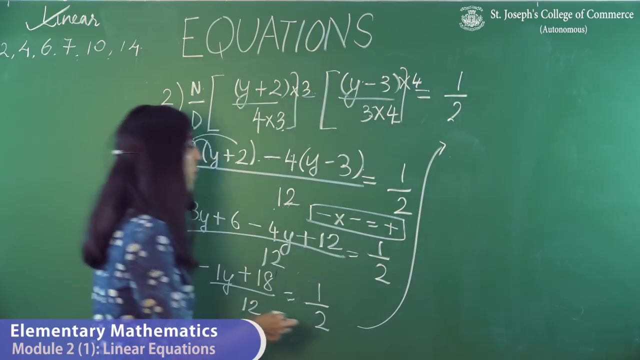 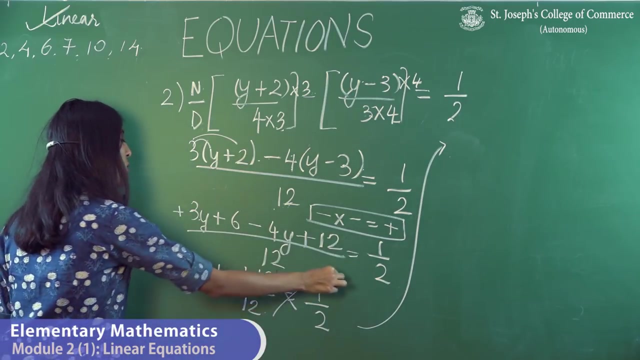 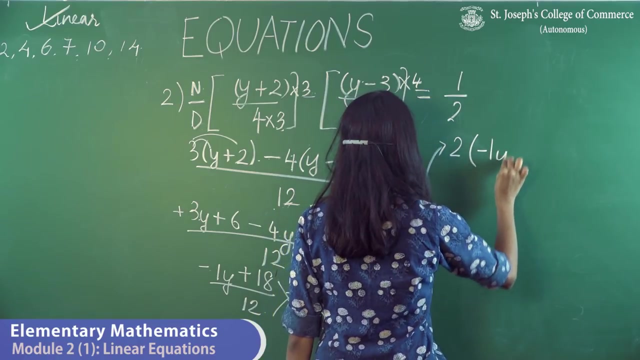 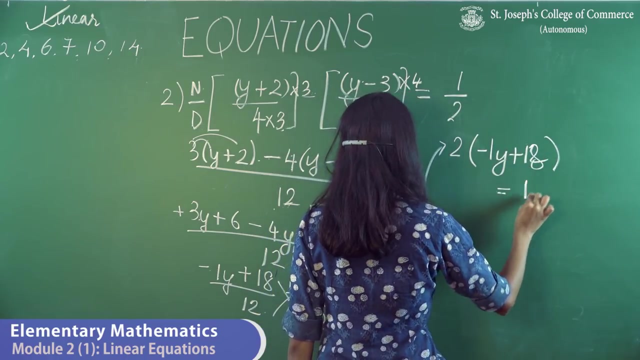 When we solve the remaining, after it's been simplified to the simplest form, you need to cross multiply it. When you cross multiply it, the 12 goes to the right hand side and the 2 is multiplied with the left hand side. So when you do it, it will be 2 into minus 1y plus 12 plus 18, sorry- is equal to 12 into 1.. 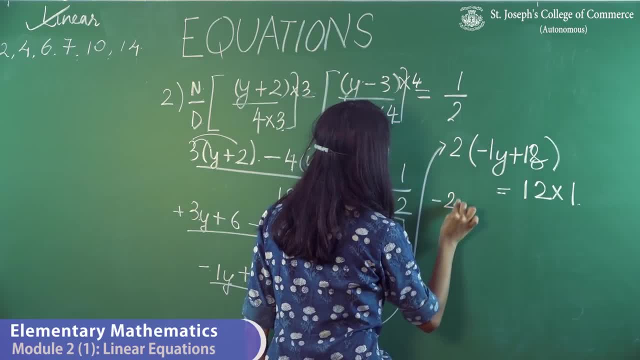 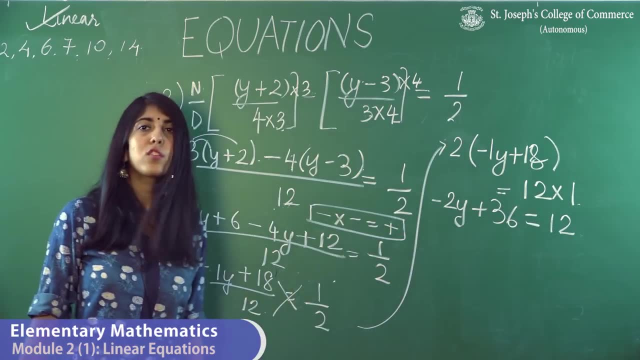 2 into minus y is equal to minus 2y. 2 into 18 is 36.. 36 is equal to 12.. When you solve it, you need to transfer all the variables to one side and all the constants to the other side. 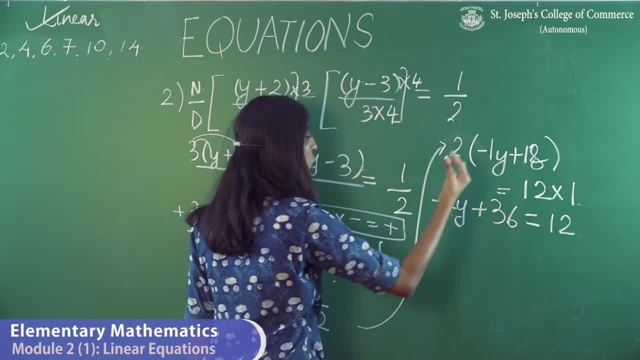 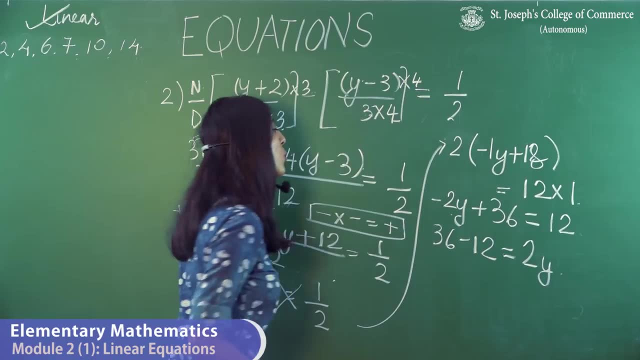 Let's keep the variables on the right hand side and the constants on the left hand side. So 36 minus 12 is equal to 2y. Why I'm doing this is because 12 is preceded by a plus sign, So when it's shifted to the left hand side, it becomes minus. 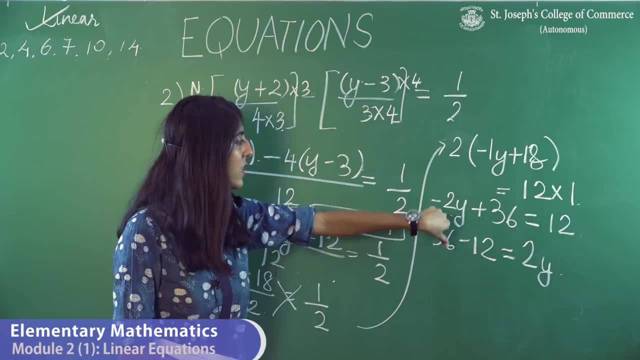 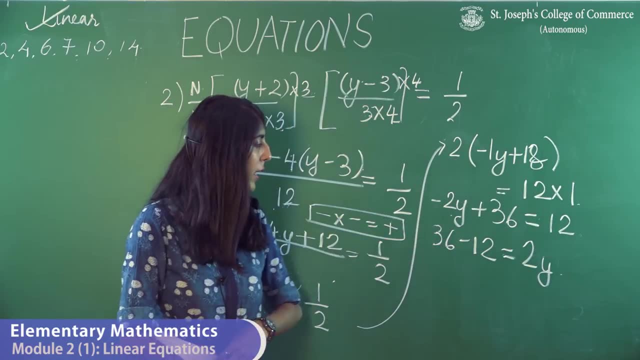 Applying the rule that I taught earlier, When 2y is transferred to the right hand side from the LHS, 2y is preceded by a negative sign, So when it's transferred it becomes plus 2y. 36 minus 12 is 24.. 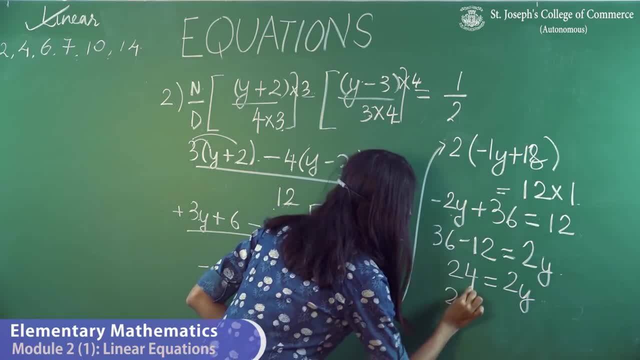 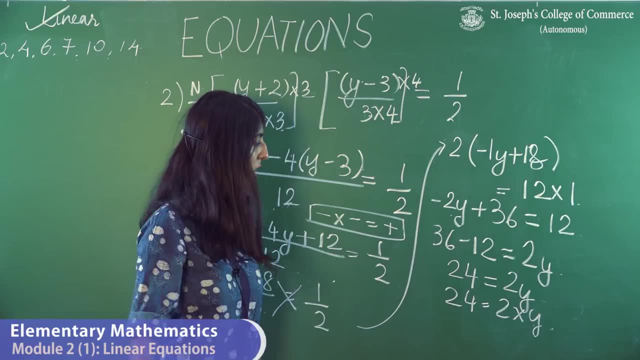 24 is equal to 2y. 24 is equal to 2 into y. So y is the variable, the answer to which we need to find out. in this equation, It is multiplied by 2.. So when 2 goes to the other side, it becomes division. 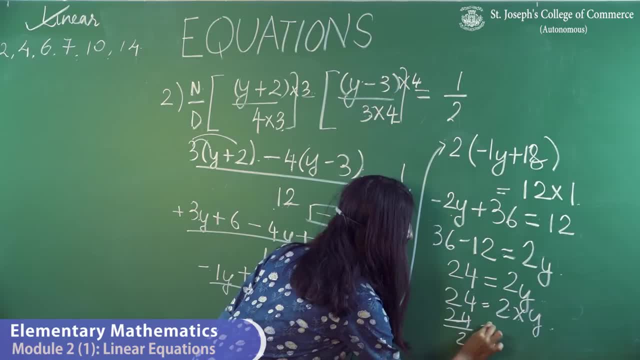 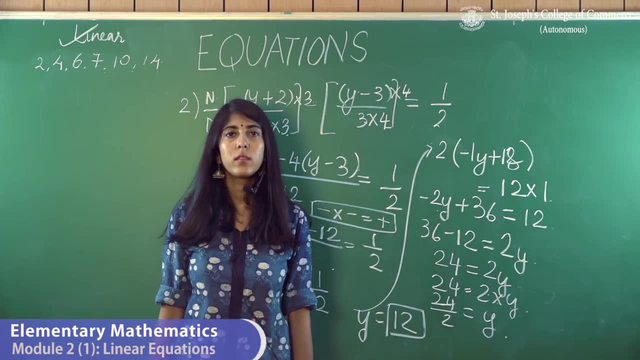 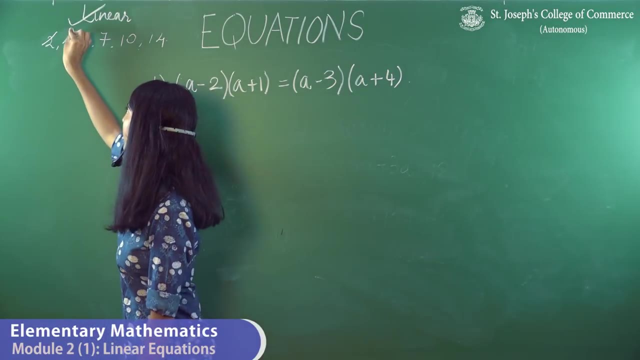 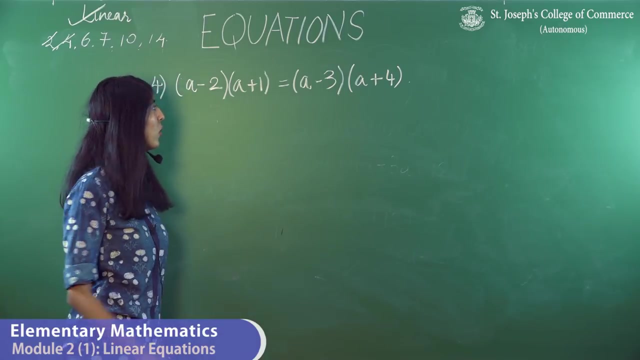 So 24 divided by 2 is equal to y. Therefore y is equal to 12.. The next question we're going to solve is the fourth sum: a minus 2 into a plus 1 is equal to a minus 3 into a plus 4.. 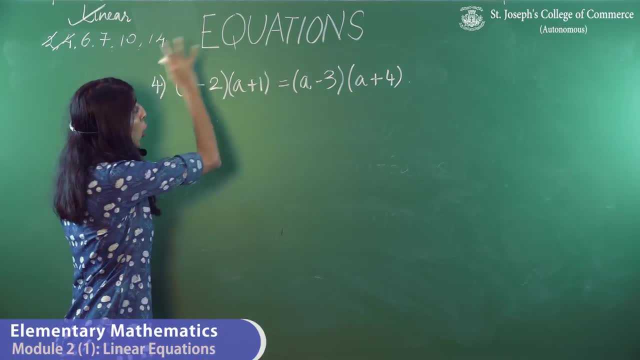 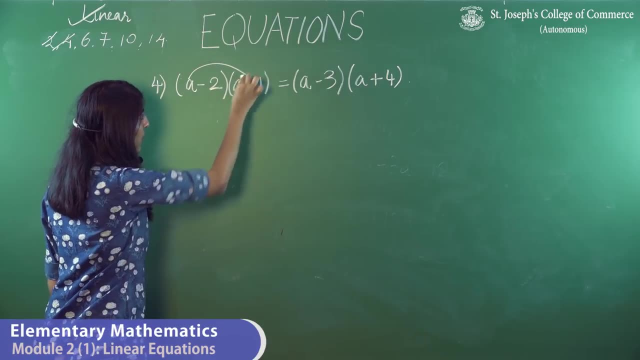 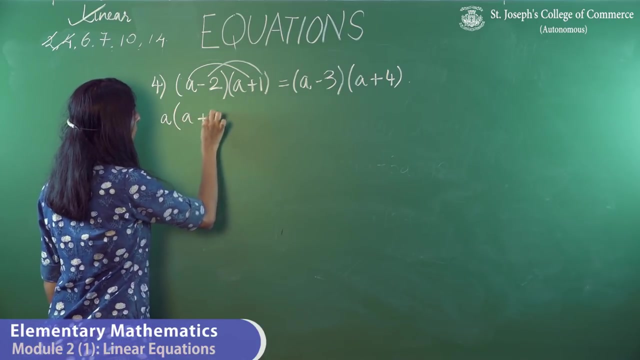 This question has a lot of brackets. We start by expanding only either of the sides so that we have a clarity on the sum. So when we start expanding, a is multiplied with this bracket and minus 2 is also multiplied with this bracket. So when we start, it's a into a plus 1, minus 2 into a plus 1.. 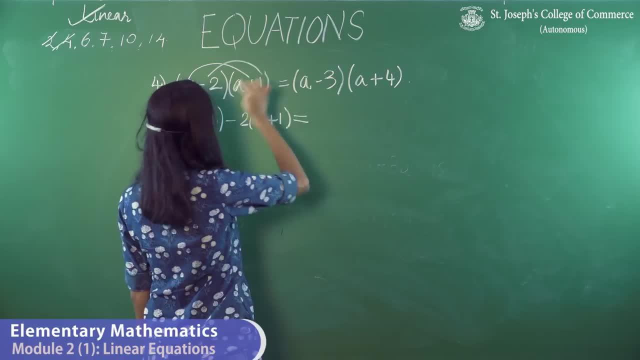 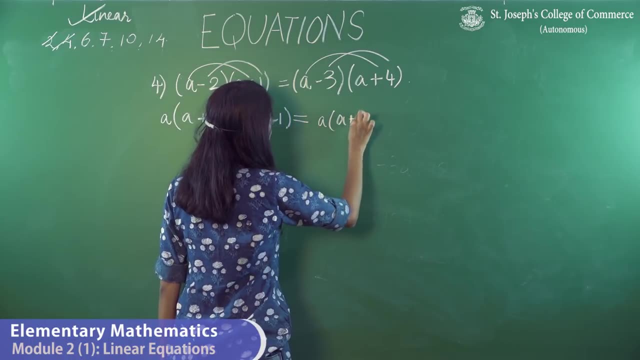 When we solve the right hand side. the same rule applies a into a plus 4 and minus 3 into a plus 4.. So a into a plus 4.. And minus 3, do not forget the minus sign- into a plus 4.. 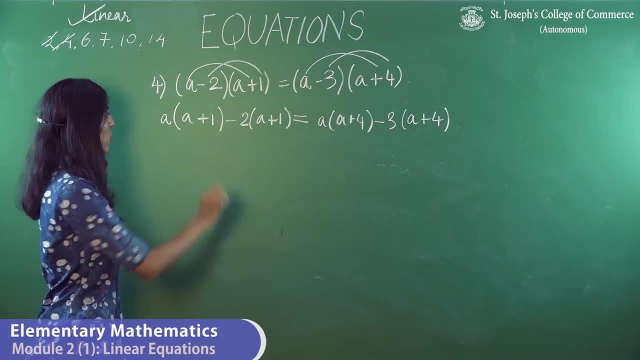 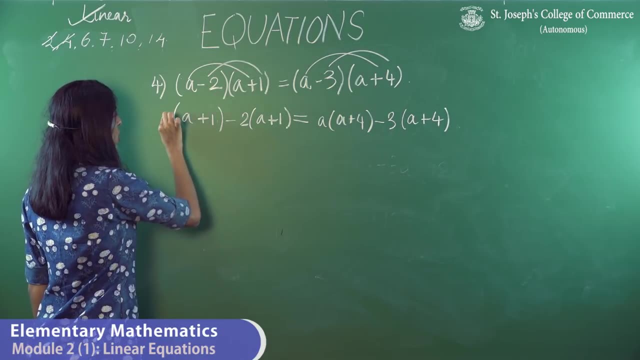 This is the first step. Now we have more clarity on the question. So now we can start expanding on the brackets. So when we expand the brackets, a is multiplied with the whole bracket. So a into a is a square and not 2a. 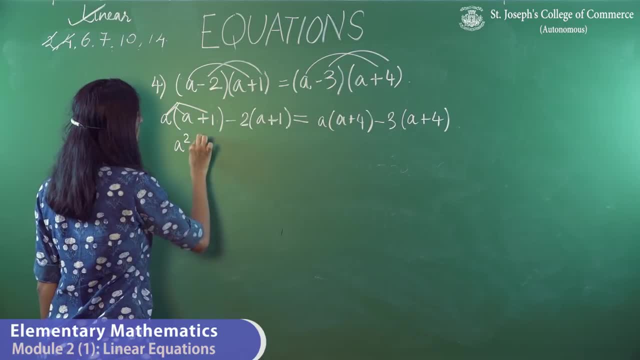 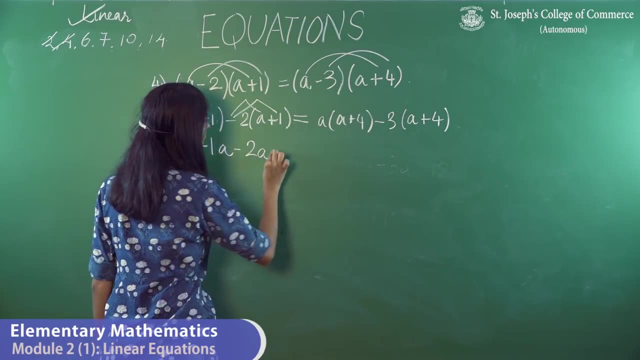 a into a is always a square. a into 1 is plus 1a. Minus 2 into a is minus 2a And minus 2 into 1 is minus 2.. Now we solve the right hand side. a into a is also equal to a square. 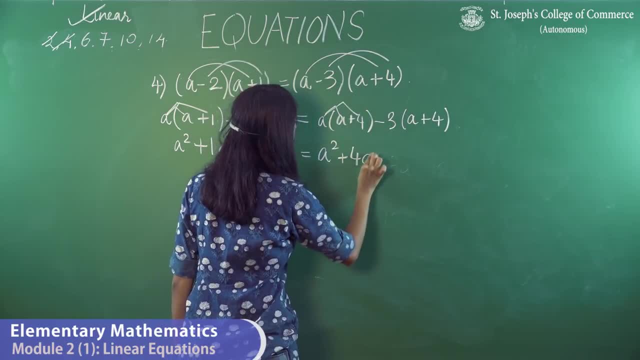 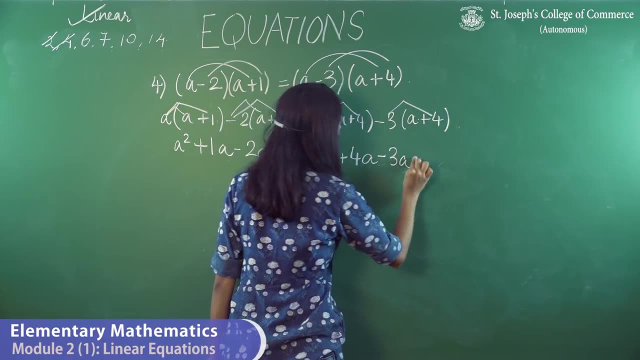 And a into 4 is equal to plus 4a. Minus 3 into a is minus 3a, And minus 3 into 4 is minus 12.. Now that we have received this, this is the simplest form of the equation. 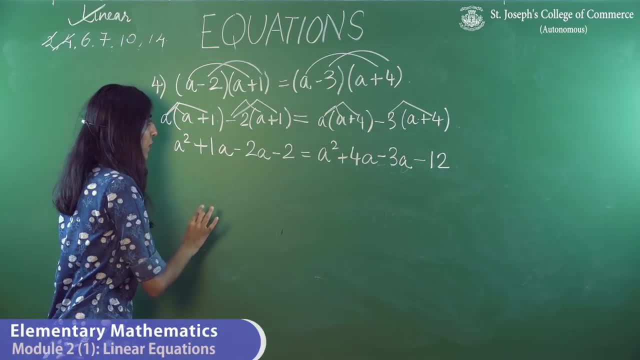 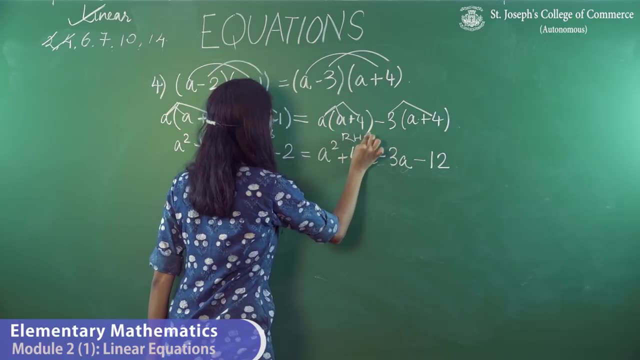 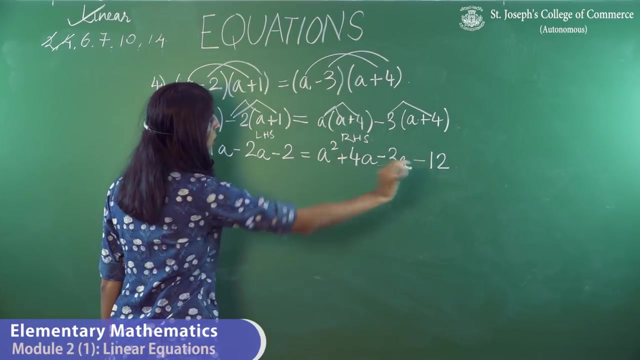 Now we need to transfer all the constants on one side of the equation And all the variables on the other side. So this is the LHS and that is the RHS. Let's start by transferring all the a's on LHS and all the constants on the RHS. 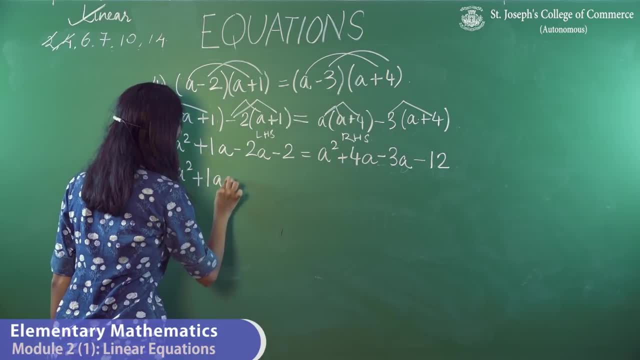 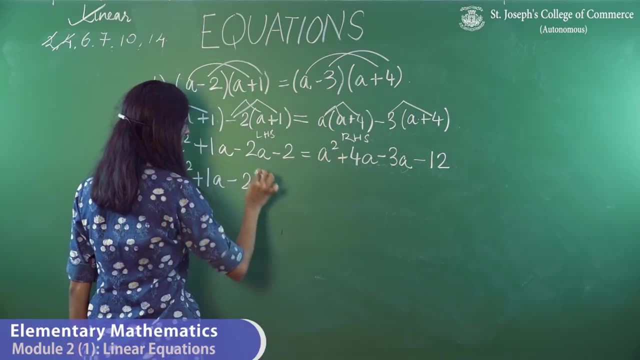 So all the a's remain as it is on the LHS, as it is a square plus 1a, minus 2a. When we shift a square to this side, it is preceded by a plus sign. So when we shift it to the other side, it does not change. 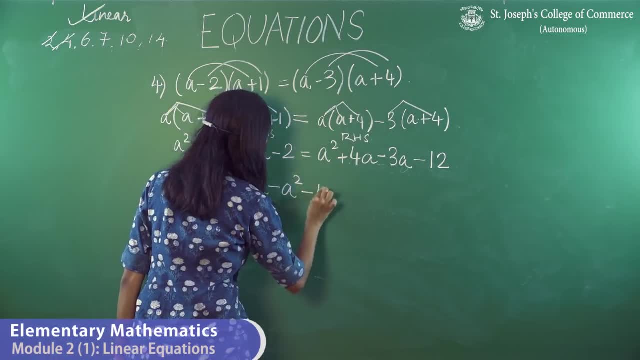 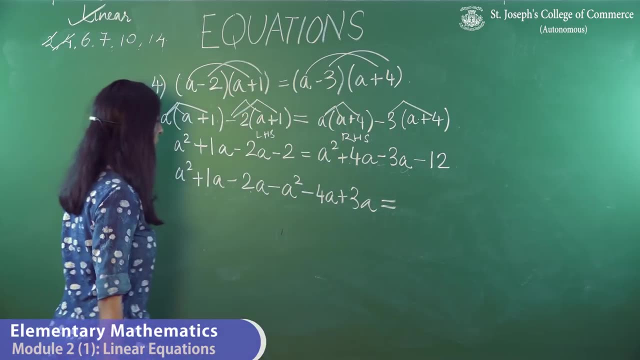 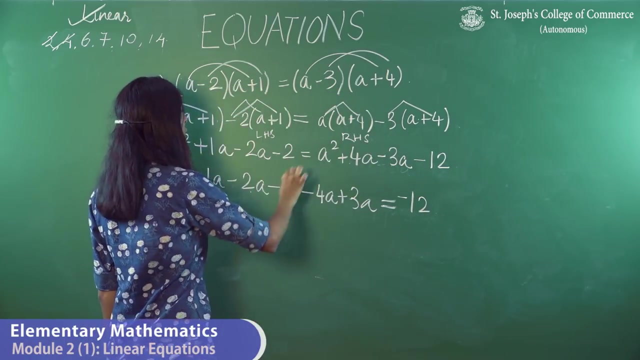 It becomes minus. Plus 4a also becomes minus 4a, And minus 3a will become plus 3a. The other side of the equation already has a minus 12.. So let's leave this as it is, And the only constant on the LHS was minus 2.. 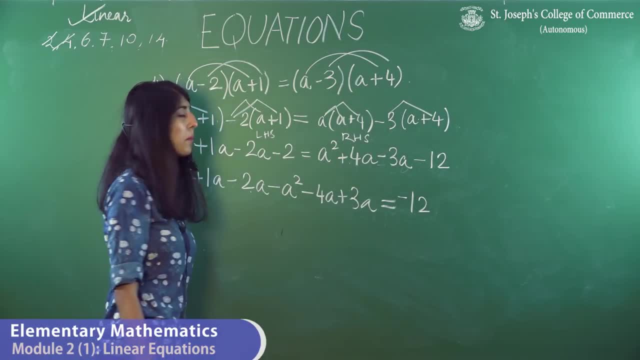 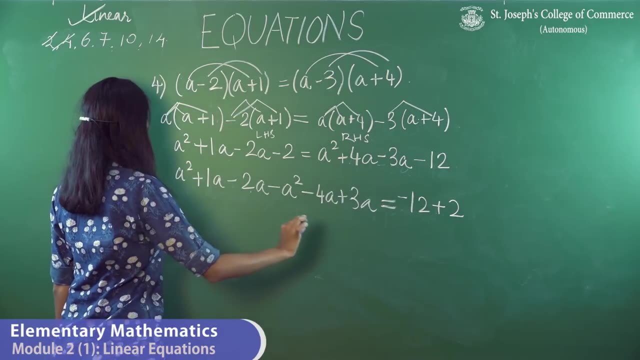 2 is preceded by a minus sign, So when it is shifted to the other side, it becomes plus 2.. So minus 12 plus 2.. Now that we have come to this part of the equation, you need to cancel out the answers. 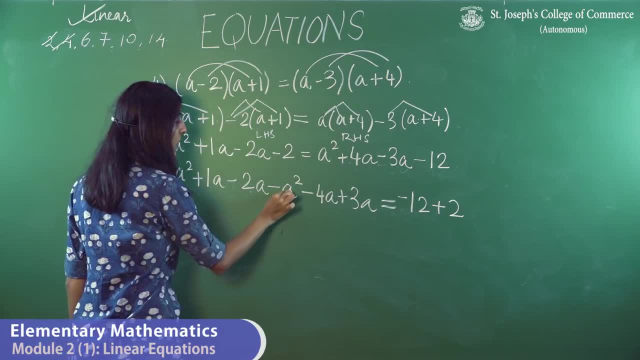 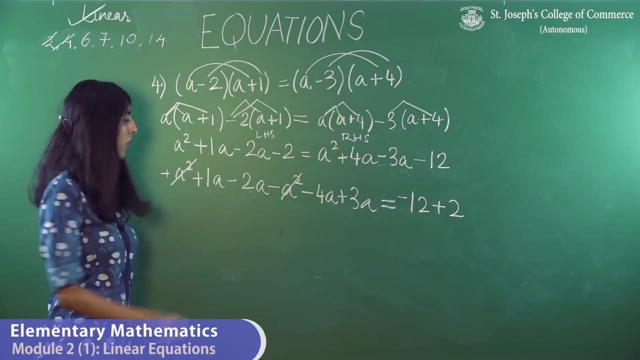 So if you notice plus a square and minus a square have the opposite signs On the number line, when you solve it you get a zero. So you cancel out these two values. Then you solve it using BODMAS. You first a, comes first and only then s. 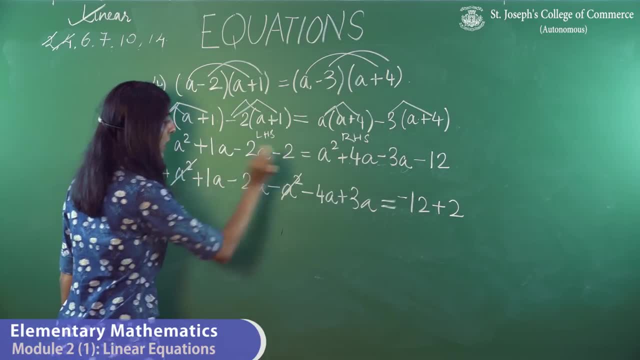 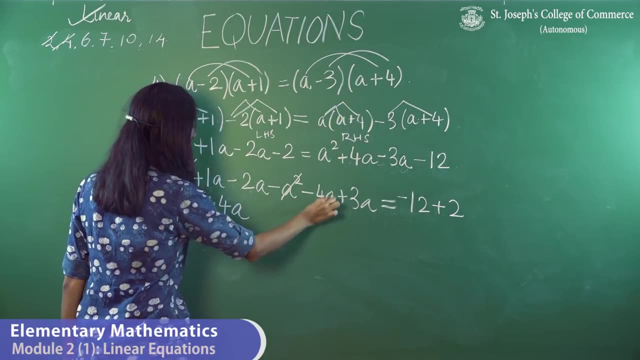 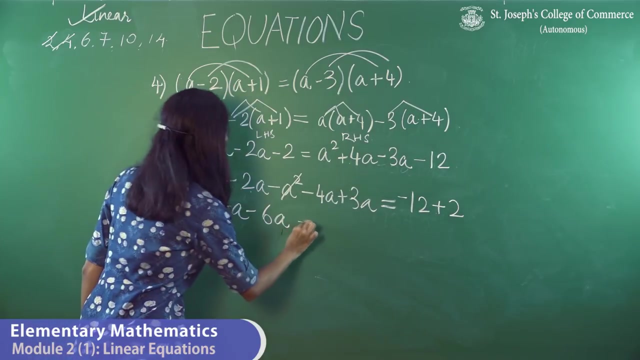 So you first add the variables. So plus 1a, plus 4a- I mean plus 3a- will give you plus 4a, And when you do minus 3a you get 0. And when you do minus 2a and minus 4a you get minus 6a. 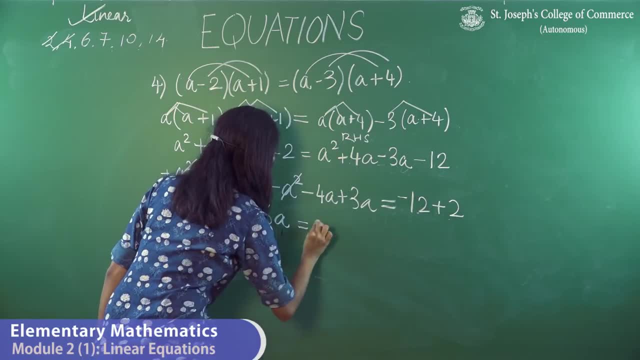 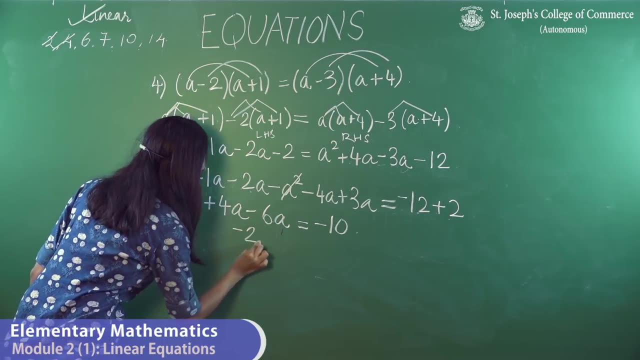 The other side remains minus 12 plus 2 will give you a minus 10.. Okay, When you solve it: plus 4a, minus 6a will give you minus 2a. This is because both the signs are opposite. 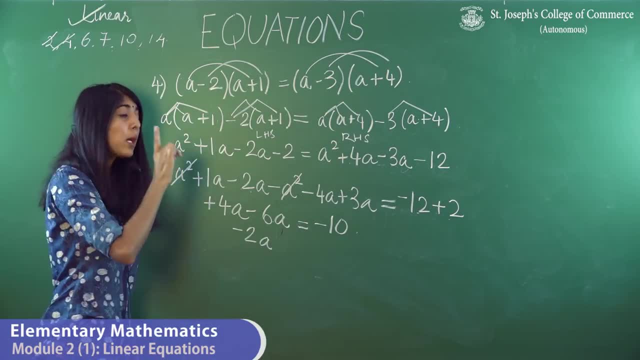 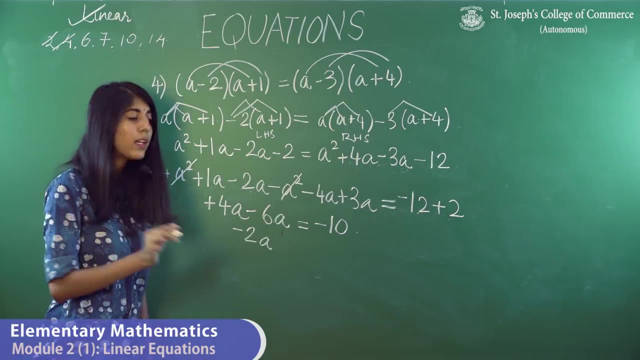 And when the signs are opposite, you need to subtract according to the number line rule that we have done before. When you subtract, you get 2a. The greater number is preceded by a minus sign and hence you write minus 2a. 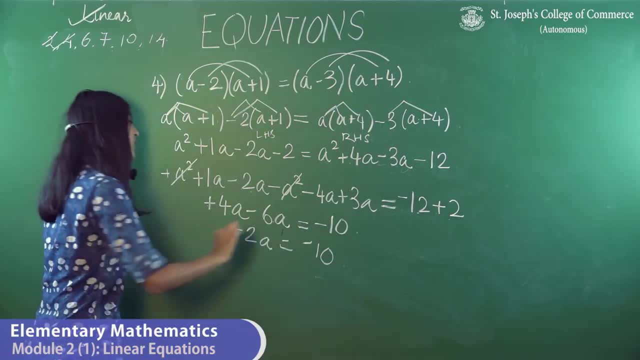 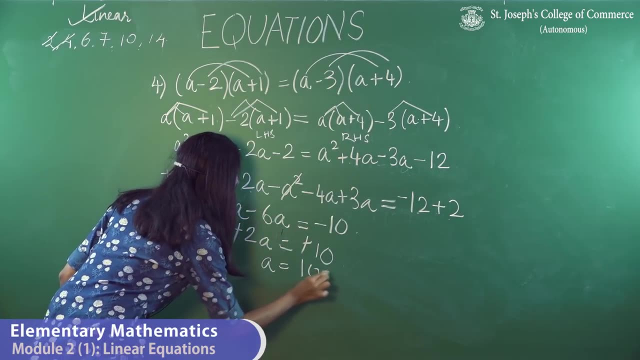 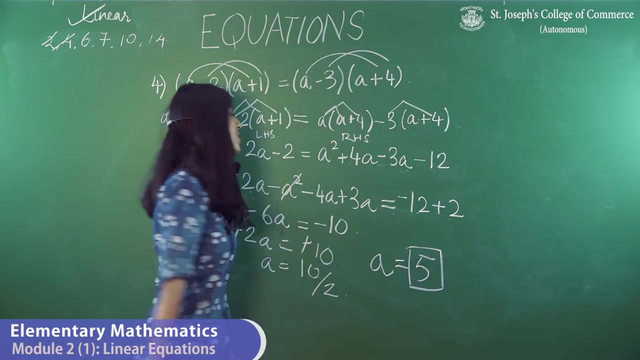 Minus 2a is equal to minus 10.. As both the sides of the equation have a minus, you can cancel out the minus signs When you solve it. a is equal to 10 divided by 2.. Therefore, the answer of a in this linear equation is equal to 5.. 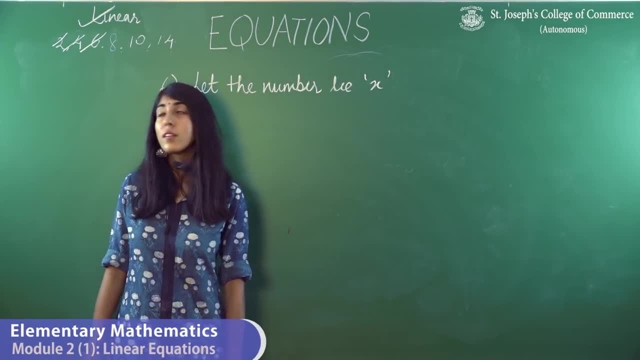 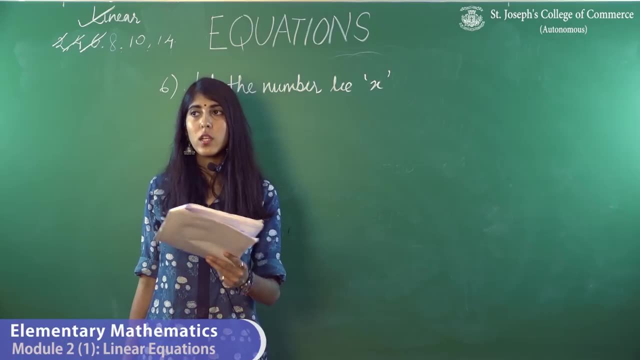 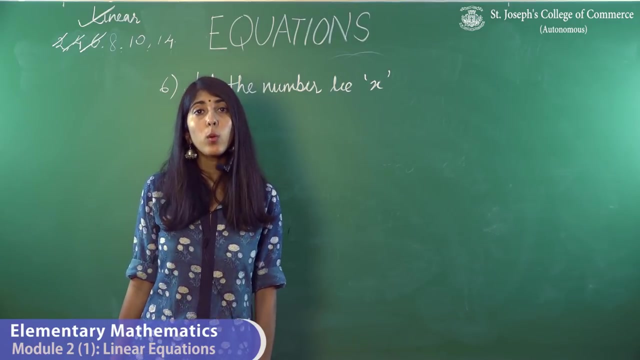 The next question we're going to be solving is the sixth sum. The sixth sum is a word problem. When we look at a word problem it says 4 times a number increased by 7 is 31.. Find the number. So every time a question says find the number or find anything, assume that number or that unknown variable to be x. 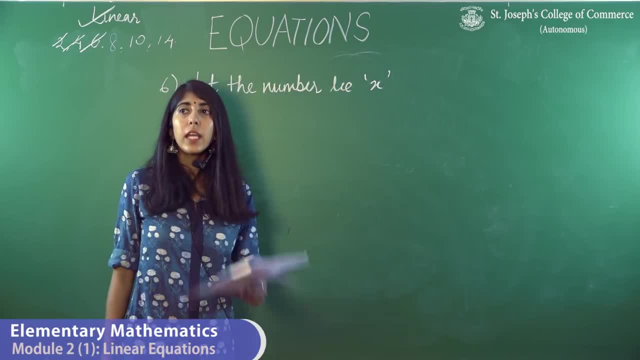 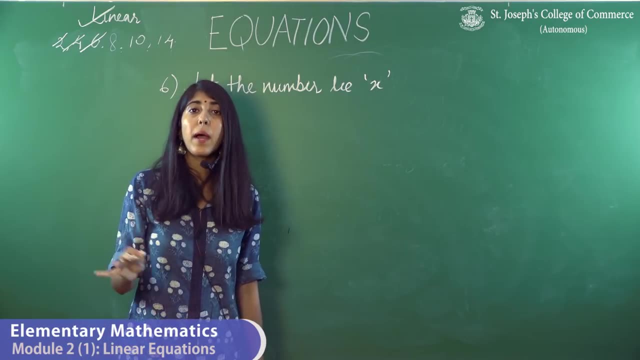 So, as you've written here, let the number be x. If you look into the question, it says 4 times a number. Any times anything is separated by a multiple. Any times anything is separated by a multiplication sign. The question says 4 times a number. 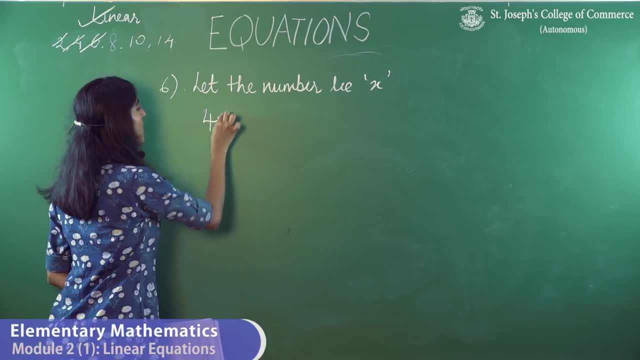 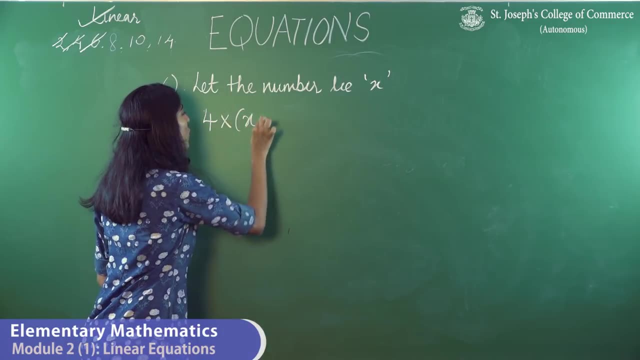 Since a number has been assumed to be x 4 times is separated by a multiplication sign. So 4 times a number means 4 into that number. So 4 into that number increased by 7.. Increased by 7 means 7 is added to that equation. 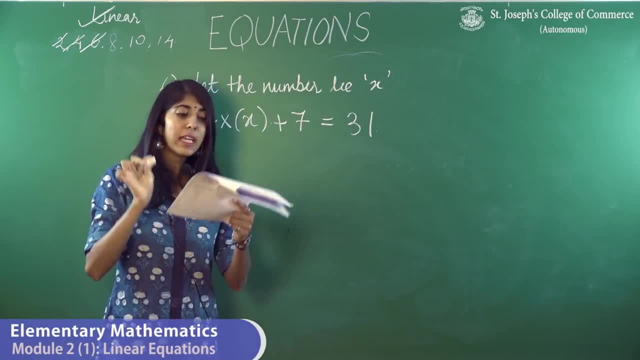 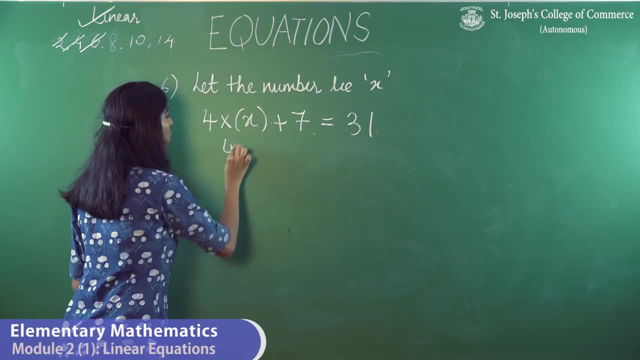 So 4x plus 7 is equal to 31.. When they say is 31, is is assumed to be an equal to sign. So 4 into x plus 7 is equal to 31.. So when we solve it you get: 4x plus 7 is equal to 31.. 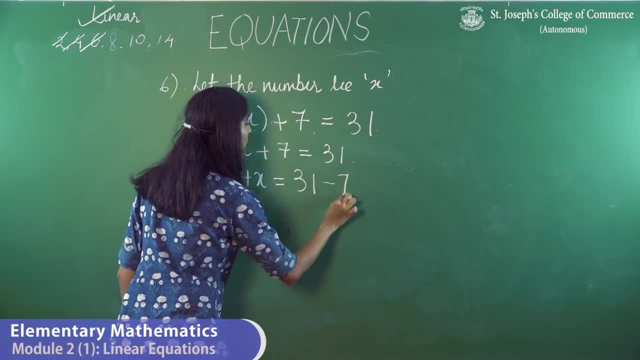 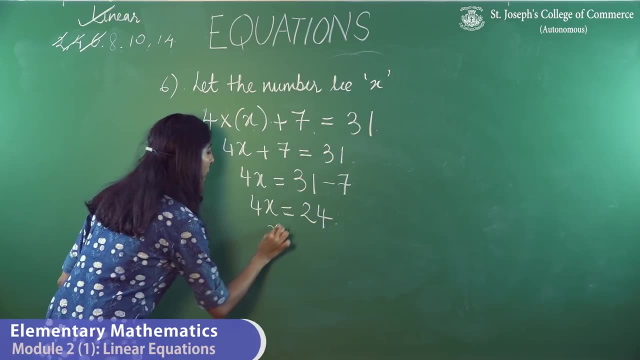 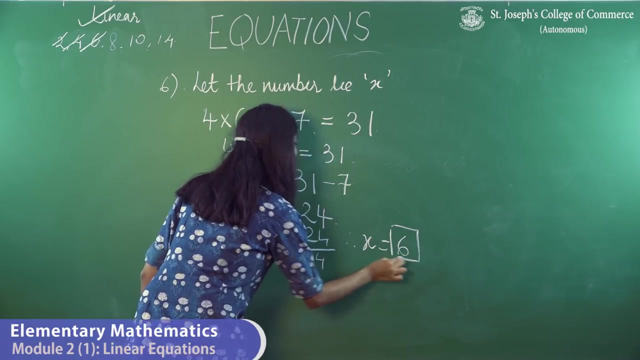 4x is equal to 31 minus 7.. 4x is equal to 24.. x is equal to 24 divided by 4. And therefore x is equal to 6.. Don't forget, once you find the value of the unknown variable. 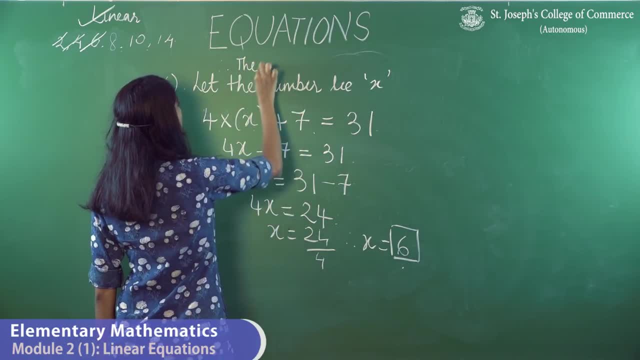 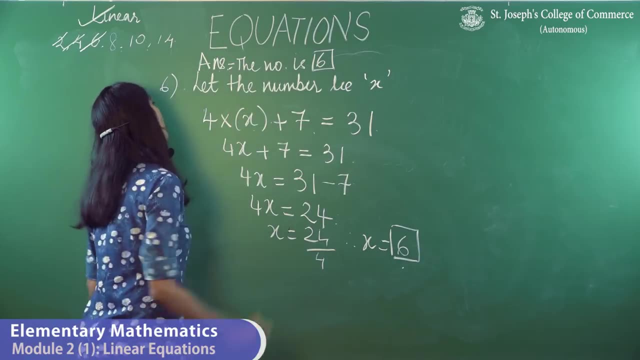 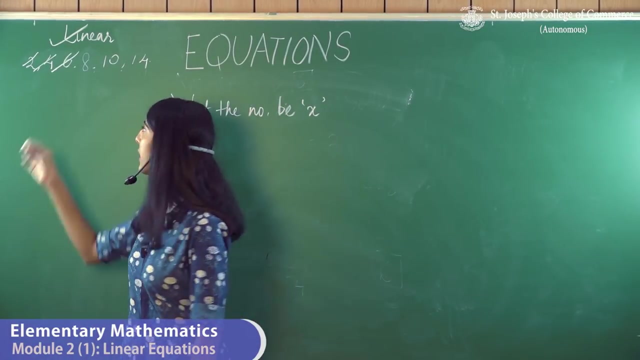 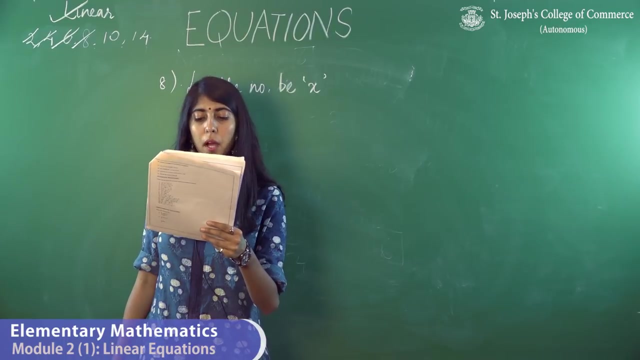 make sure you write: therefore, the number is 6.. This is how you end the question. The next question we are going to be solving is the 8th question. The 8th question says: if the 4th part of a number exceeds its 6th part by 5,. 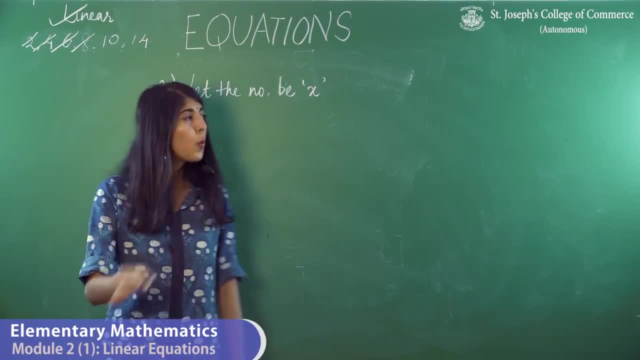 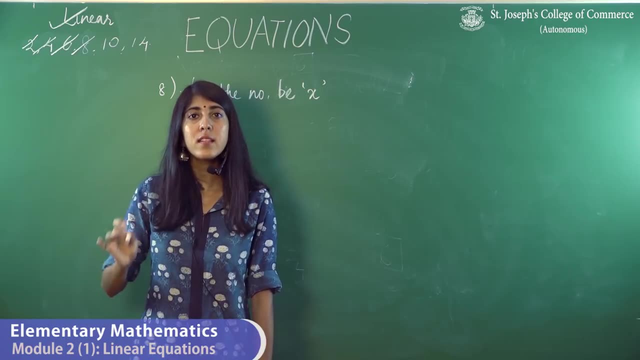 find the number. Since it says find the number, we start off by assuming the number to be x. If anything is 4th part or 6th part, that means it is 1 by 6 or 1 by 4.. 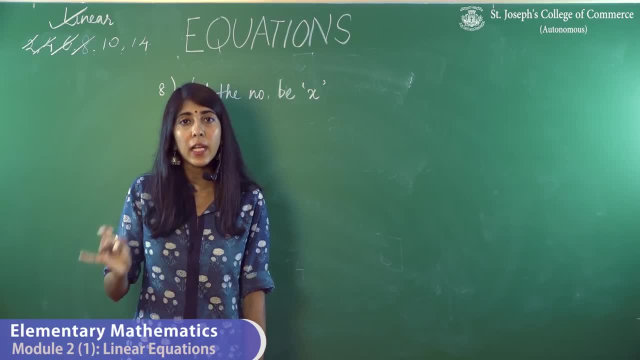 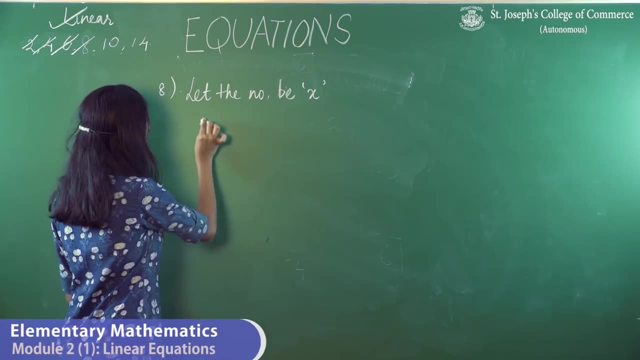 That means if I have a pie and I say I'm dividing it into 8 parts and I say I want the 7th part of it, that means it's the 1 by 7th part of it. The same way, if I say 4th part, it is x by 4.. 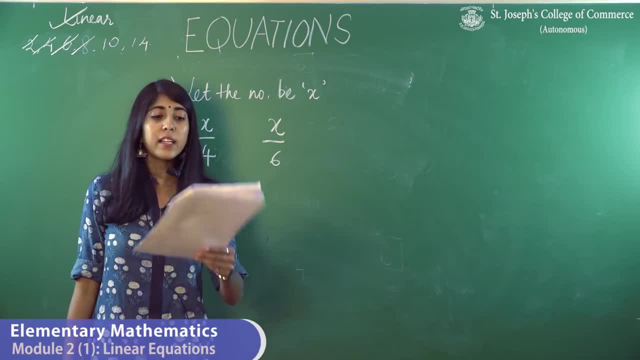 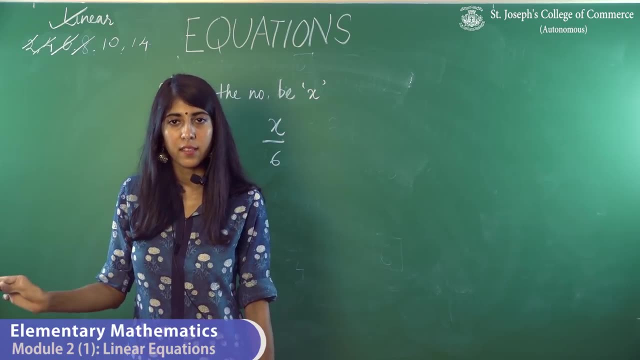 And if I say 6th part, it's x by 6.. Let's try to understand the framing of the equation. It says if the 4th part of a number exceeds its 6th part by 6.. By taking another example, if I say 10 exceeds 6 by 4,. 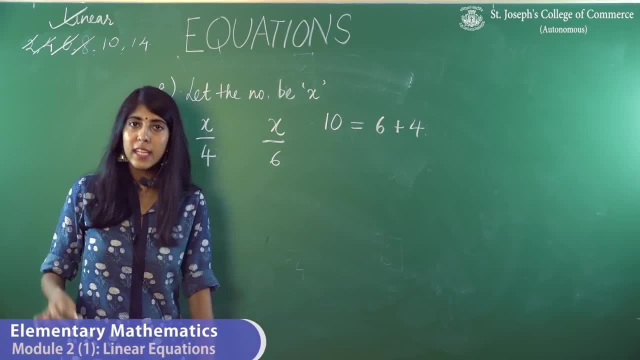 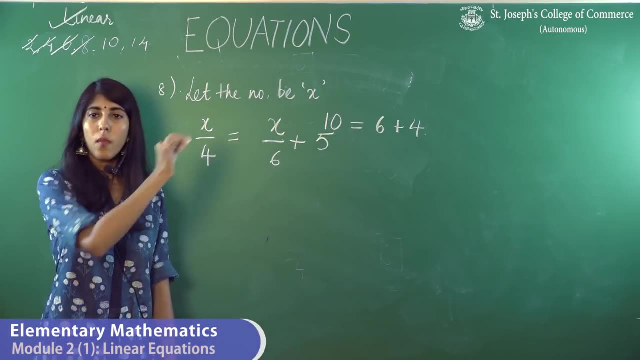 that means 10 is equal to 6 plus 4.. Same way, when I say 4th part of a number exceeds its 6th part by 5, this is the equation that you form, So it is in a fractional form. 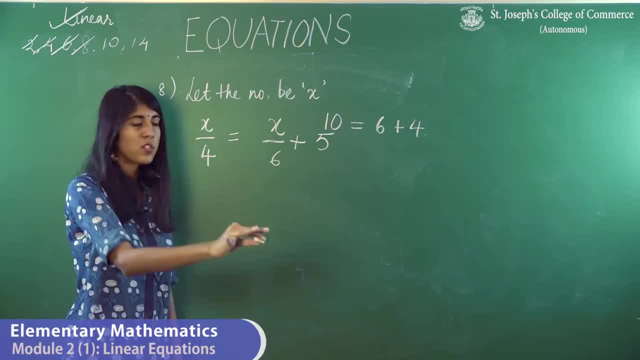 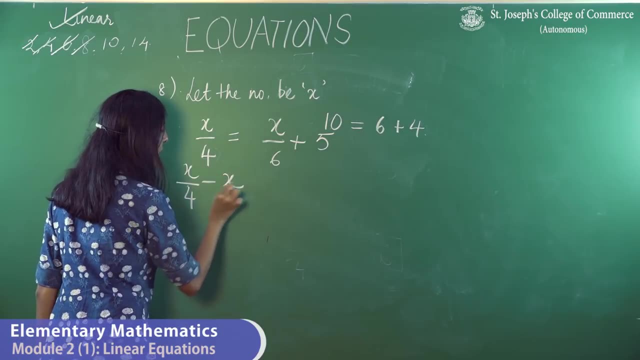 So first I do is shift all the variables to one side and keep all the constants to the other. So I shift x by 6 to the LHS, So it will become x by 4 minus x by 6 is equal to 5.. 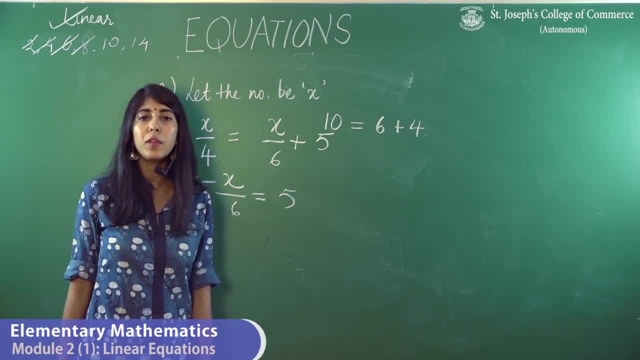 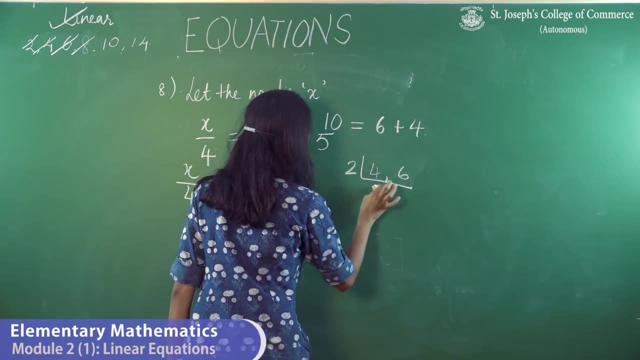 When there is a numerator and denominator involved, you need to solve it by finding out the LCM of it. When I find out the LCM of 4 and 6, you start off with 2.. Then you try 2 again. 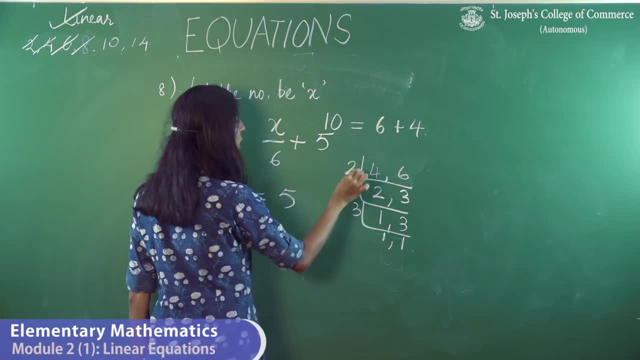 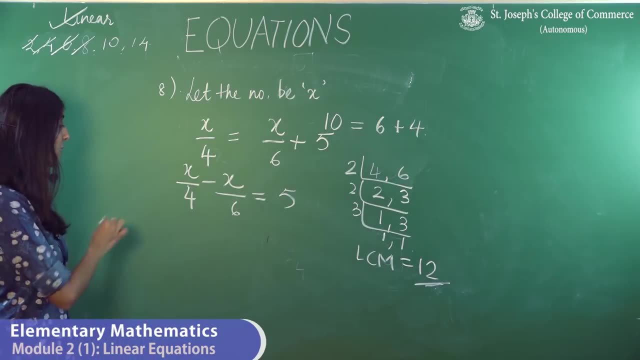 And then 3.. So the LCM will be 2 into 2 into 3, which is equal to 12.. The LCM is 12.. So you directly write the LCM as 12.. When the LCM is 12,. 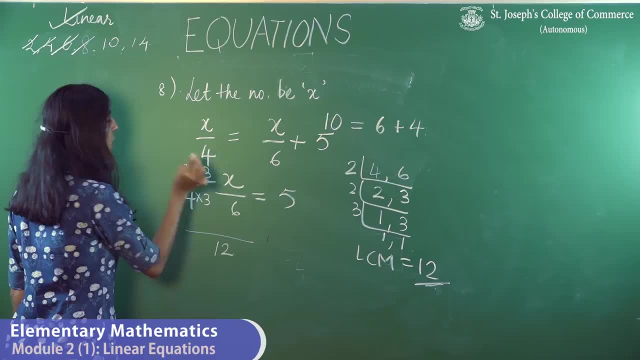 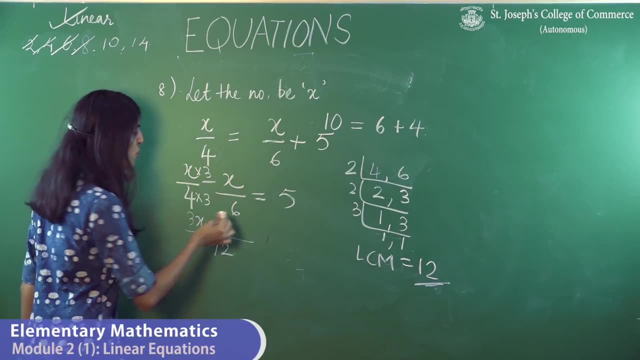 4 into 3 will give you 12.. So you multiply numerator and denominator by 3.. So this becomes 3x 6 into what is 12? 6 into 2 is 12.. So 6 into 2 and x into 2.. 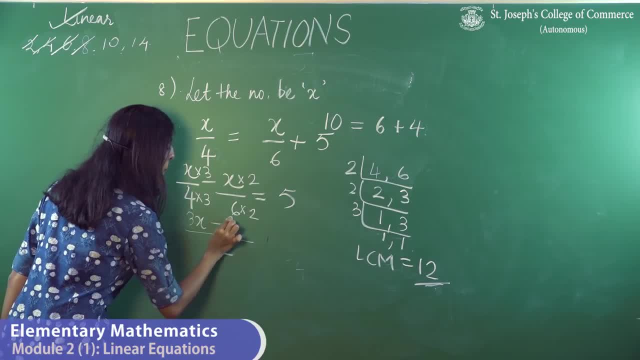 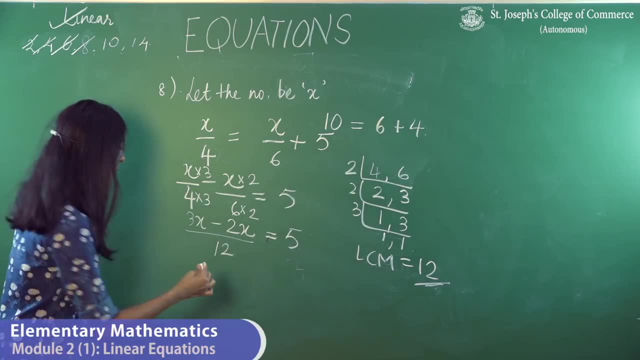 There is a minus sign that is preceding the 2.. So you do minus 2x. Leave the right hand side as it is 3x minus 2x is 1x. So 1x by 12 is equal to 5.. 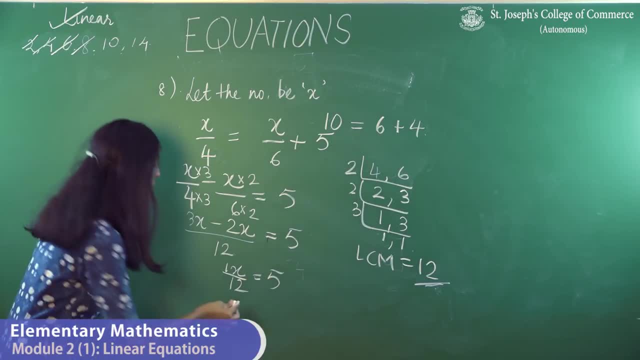 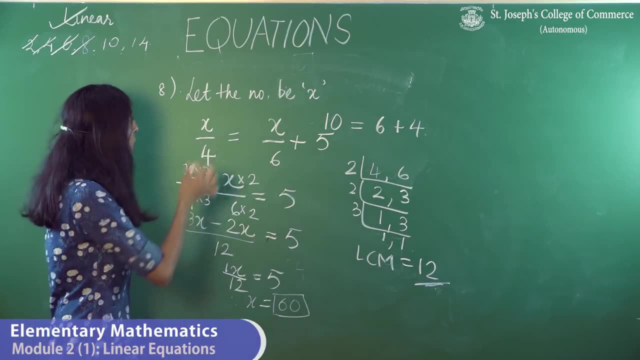 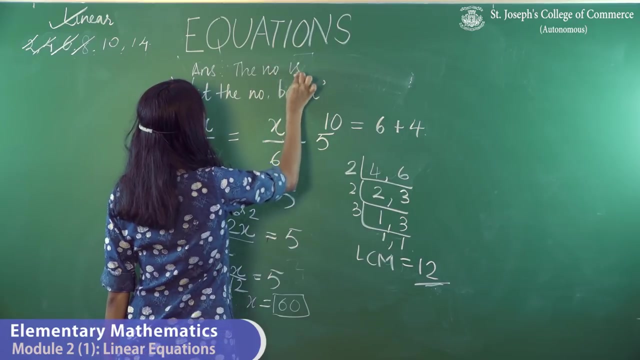 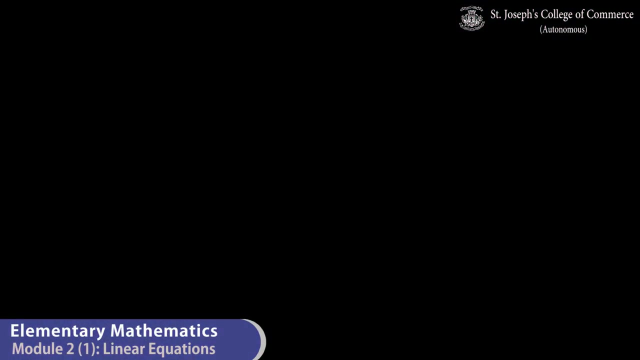 The only way of solving it is by cross multiplying. So, therefore, x is equal to 60.. Remember, this is not the answer. You need to write the answer as, Therefore, the number is 60.. The next question we are going to be looking at is the 10th question. 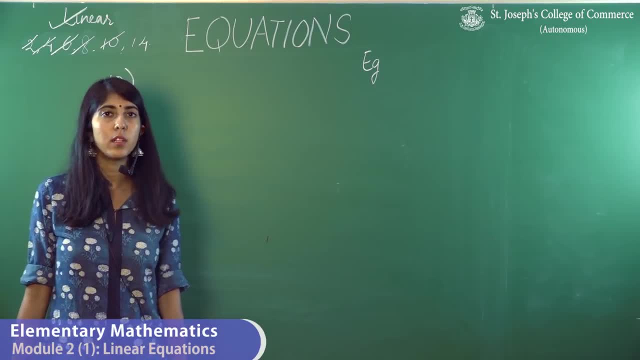 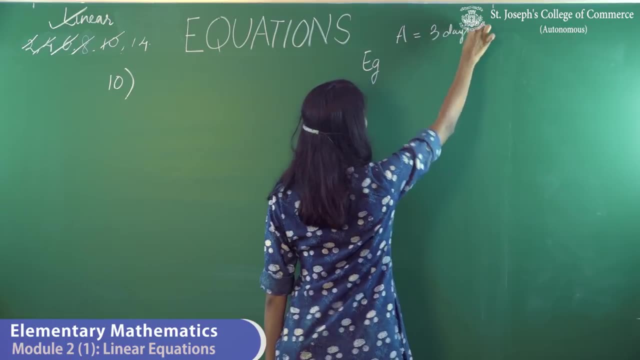 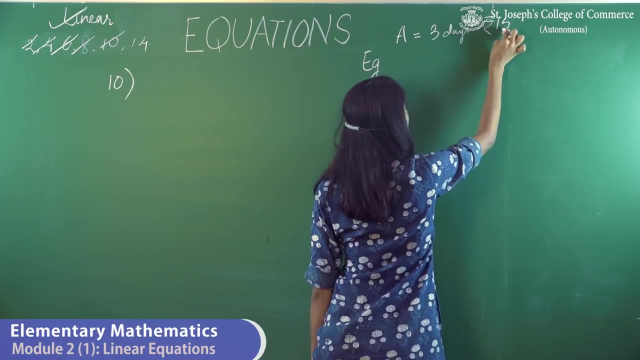 Before starting the 10th question, I am going to start with an example. Let's assume A is expected to work for 3 days in an organization. Okay, For each day that he works he is paid Rs.150.. And every day he is absent he has to give a fine of Rs.30. 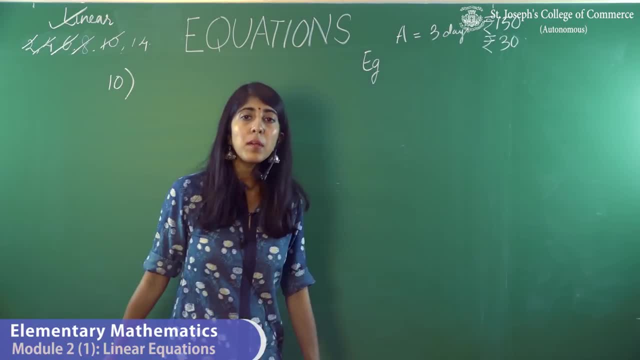 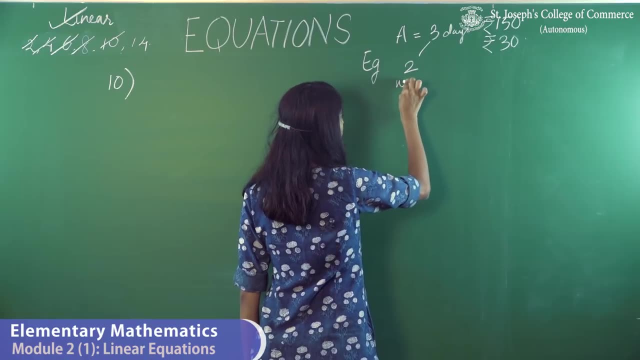 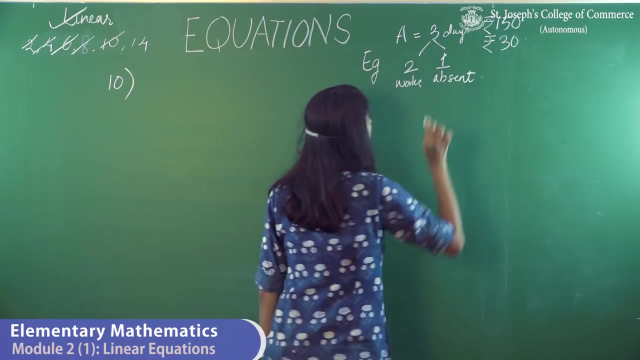 This fine will be getting deducted from his income Because you are giving it to the organization. So A is supposed to be working for 3 days, He works for 2 days and is absent for 1.. Okay, The formula that you use in this context is: 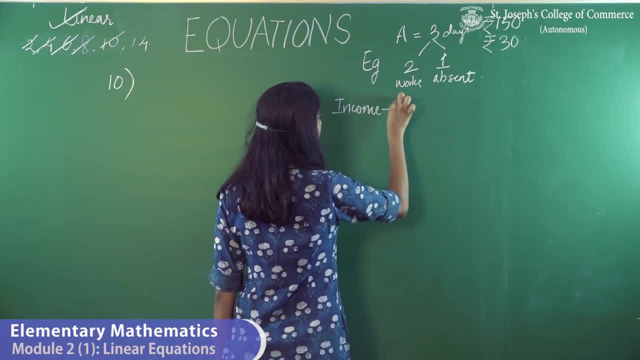 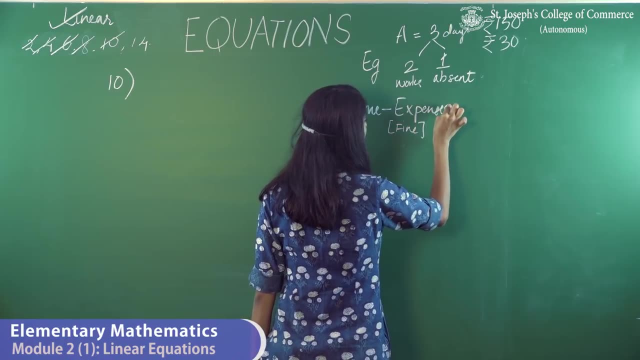 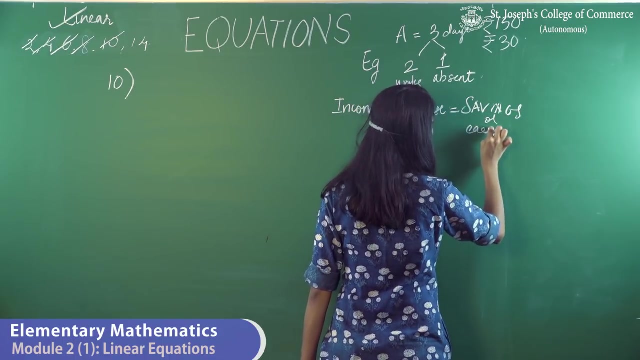 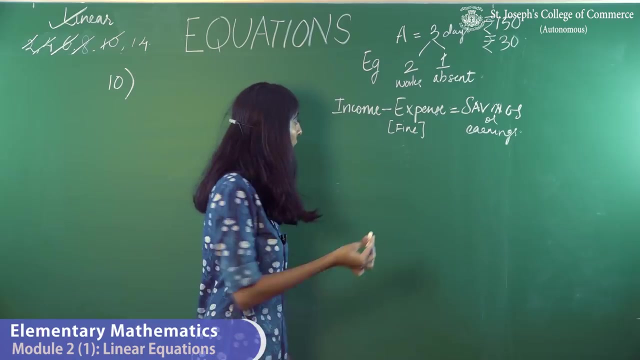 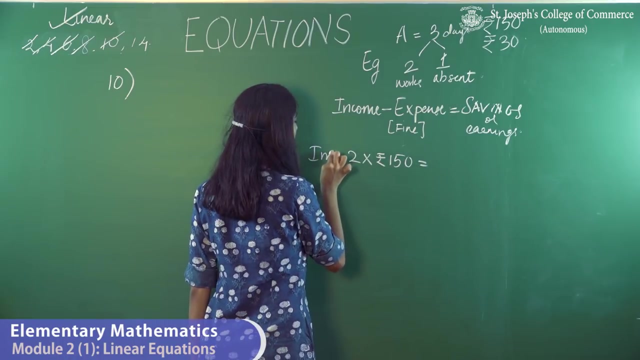 Income minus expense, which is the fine in this case, is equal to savings or earnings. In this example, since he worked for 2 days, how much does he get an income of 2 days into? Rs.150 per day, So he gets an income of Rs.300. 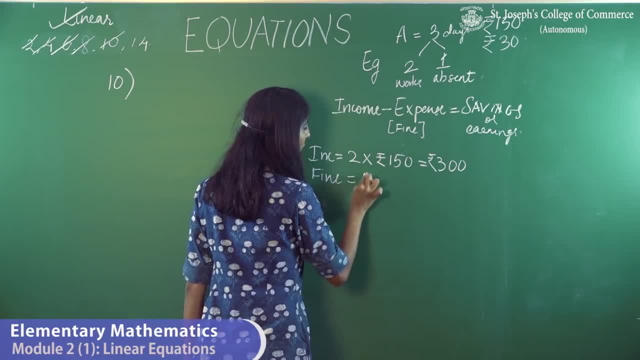 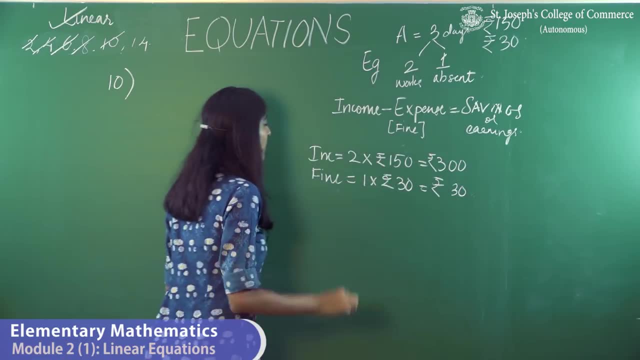 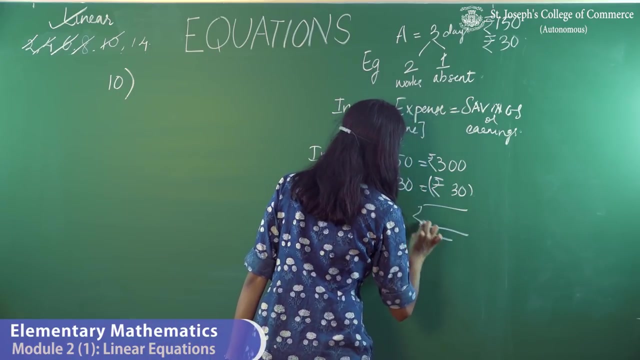 Since he is absent for 1 day, he has to pay a fine of Rs.30.. That means Rs.30 is the fine, Since your savings is income minus the fine if I deduct this from the income- your final earnings- that you get. 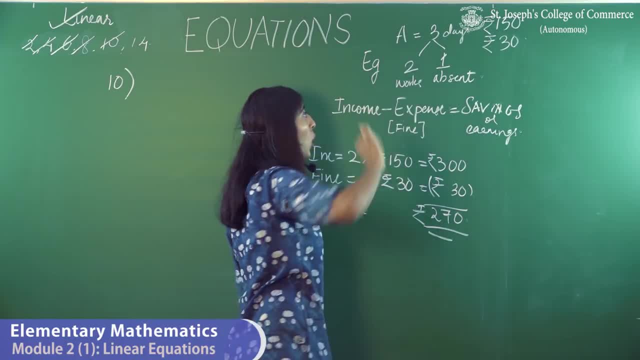 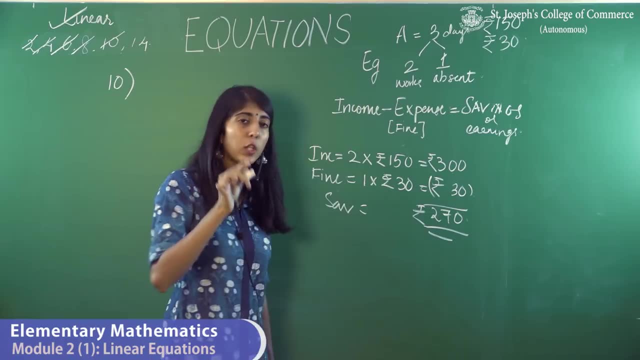 is Rs.270.. That means if he had worked for all 3 days, he would have gotten Rs.450.. Since he has worked only for 2 days, he gets Rs.300 and a Rs.30 fine is deducted from his income. 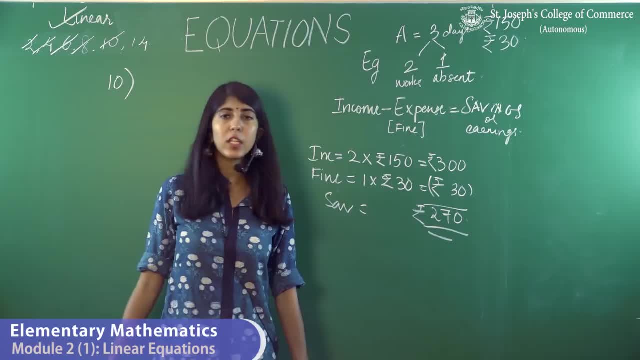 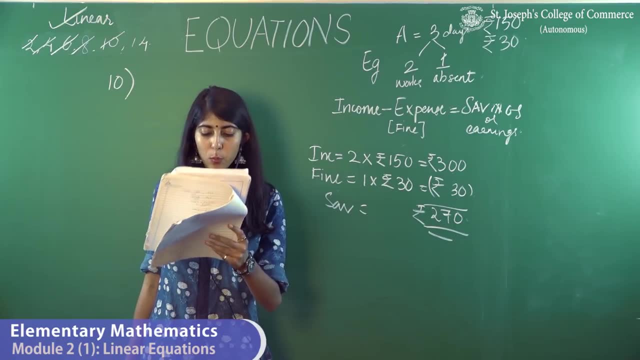 Therefore his final earnings or savings, is Rs.270.. Let's look at the question now. The question says A person is paid Rs.150 each day he worked and his fine is Rs.30 each day he remains absent. Same values. 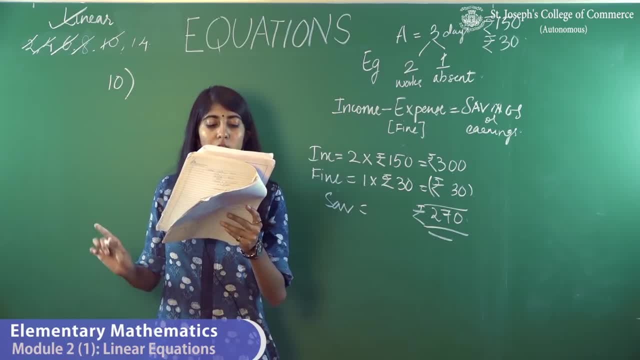 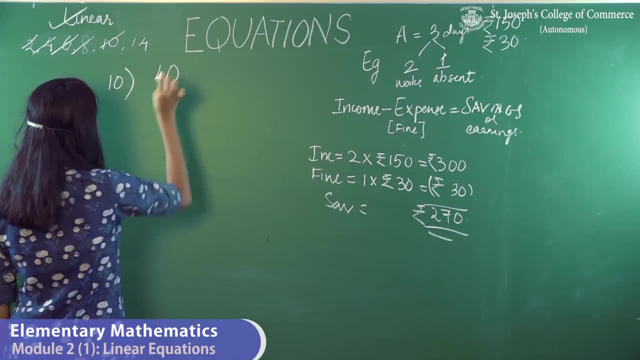 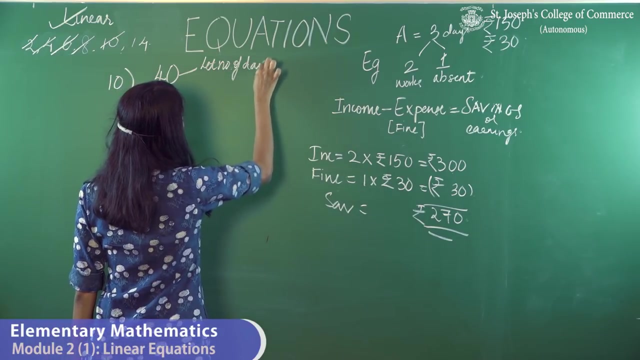 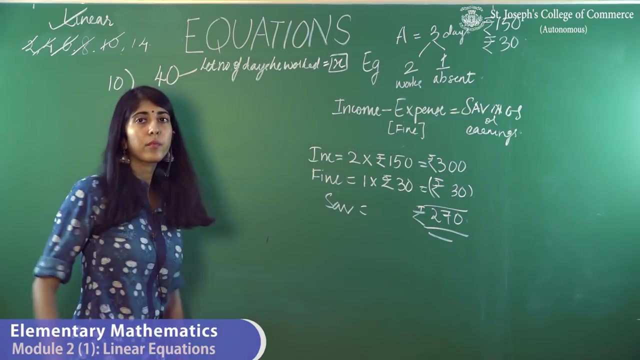 In 40 days he earns Rs.3300.. Find out how many days he worked. So the expected number of days that he is supposed to work for was 40.. Let's assume the number of days he worked for to be x. 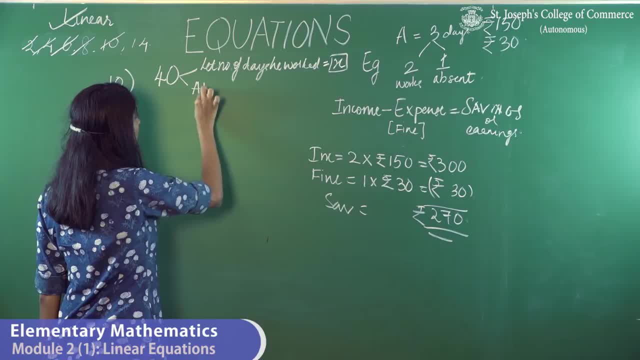 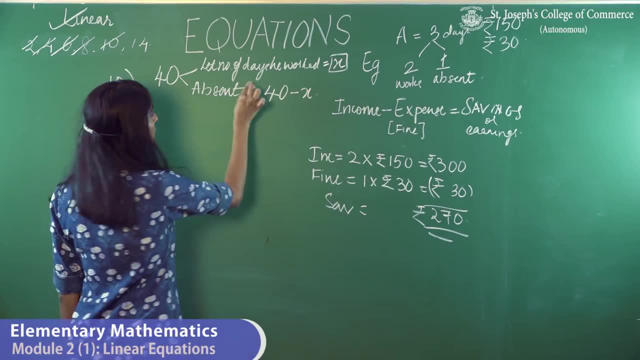 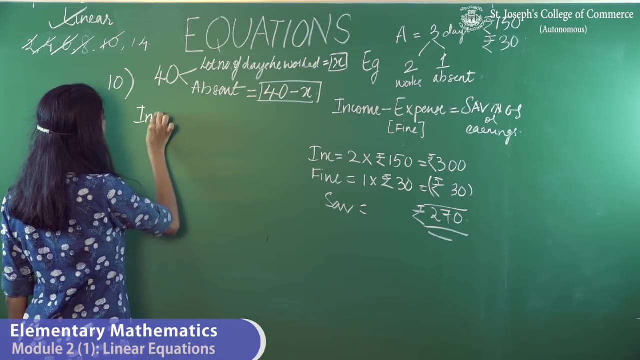 Therefore, the remaining number of days- that means the number of days he was absent for- will naturally be 40 minus x, Right? So when we continue, we understand. using the same formula that we did before. let's start writing the income of the person. 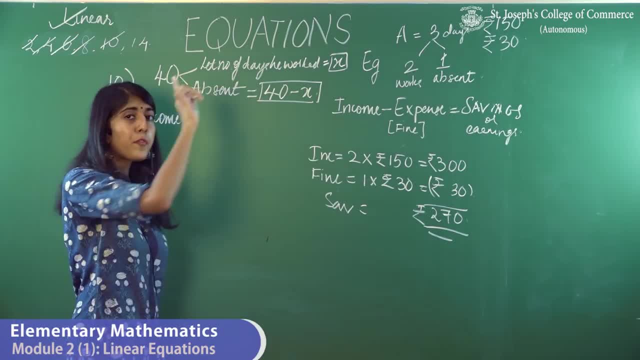 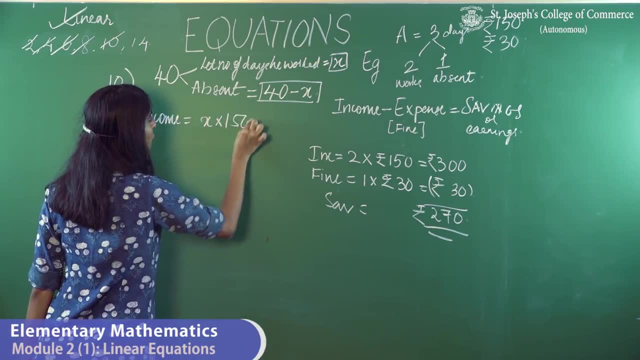 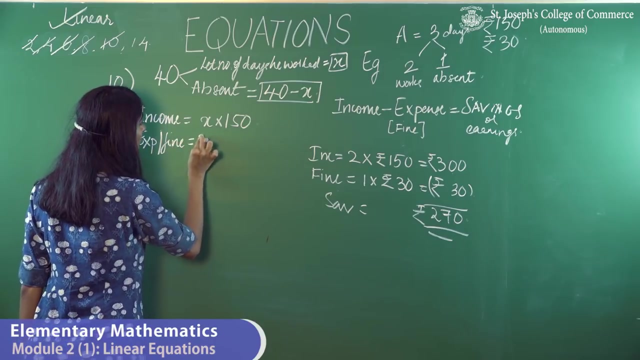 The income of the person will be Rs.150 for each day he has worked. What are the number of days he has worked for Is x, So it is x into 150.. The expense of fine is Rs.30 for each day he has been absent. 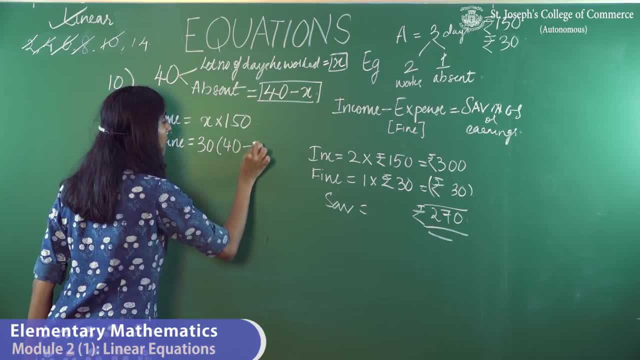 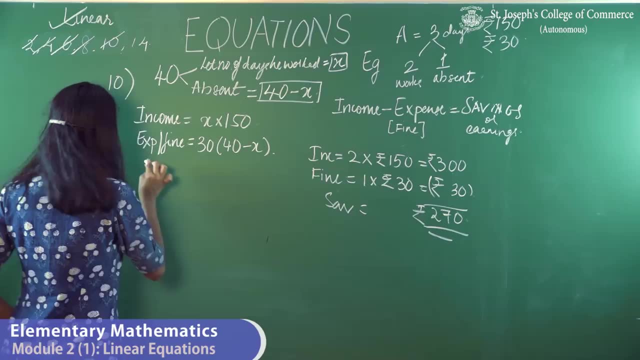 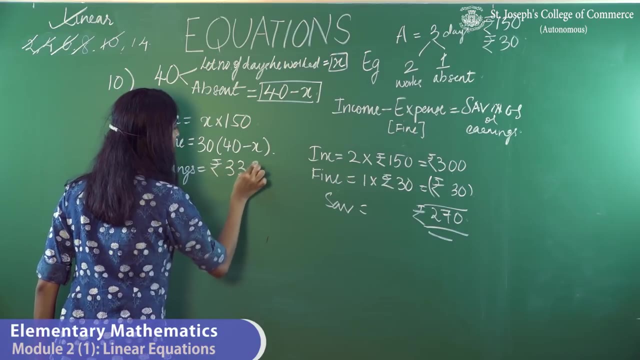 The number of days he has been absent for is 40 minus x, Right. Therefore it's been given in the question that his earnings or savings are Rs.3300.. So when you put it exactly in the form of the equation, you get. 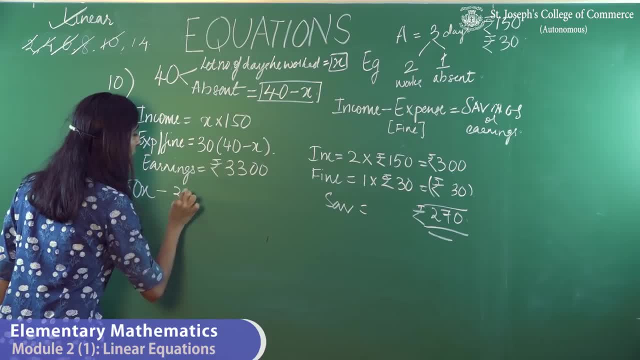 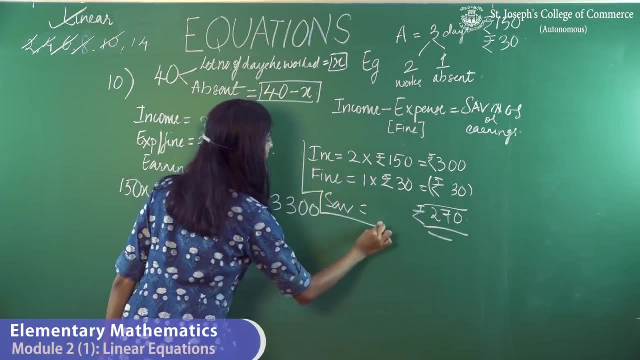 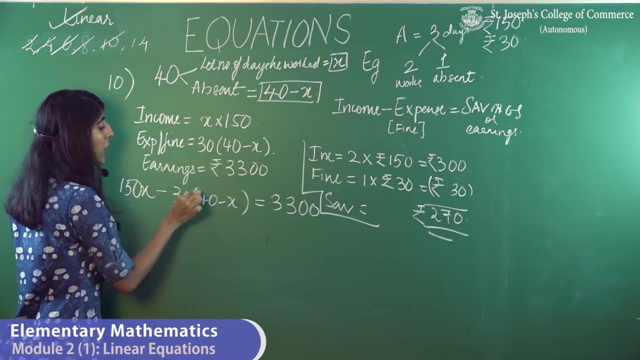 150x minus 30 into 40 minus x is equal to Rs.3300.. If you notice, income is 150x. expense of fine is 30 into 40 minus x and when you deduct the two you get your final savings. 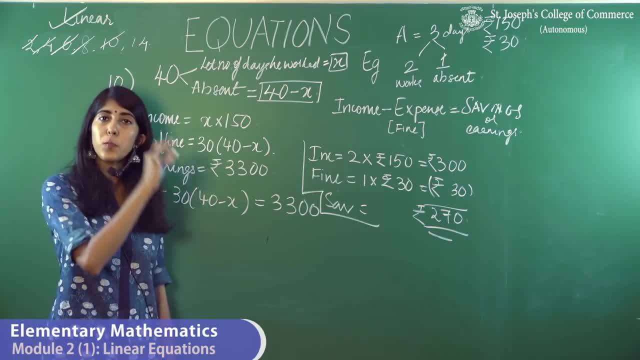 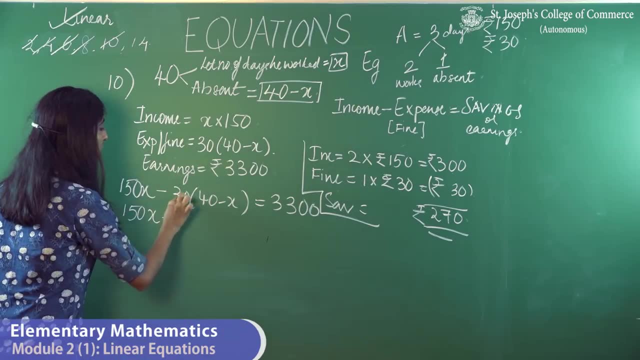 Since he has not been working for all the number of days he is expected to have worked for. When you solve the equation, you will get: 150x minus 30 into 40 is Rs.1200, minus 30 into minus x will give you. 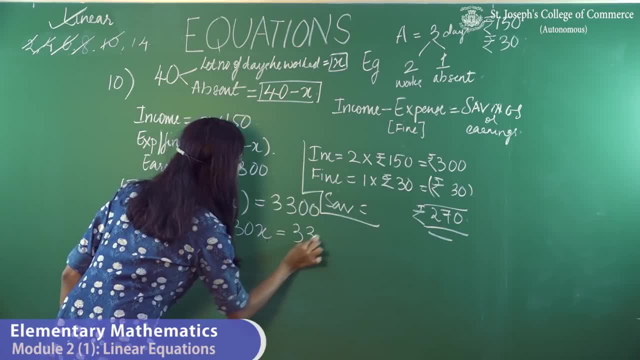 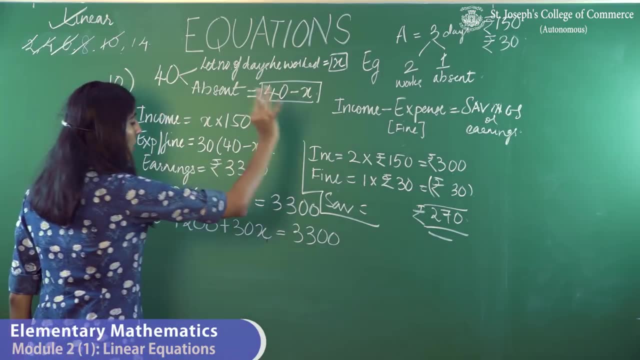 plus 30x is equal to Rs.3300.. When you solve it further, I am going to keep all the x's on this side and take the constants on the right hand side. So 150x plus 30x is equal to. 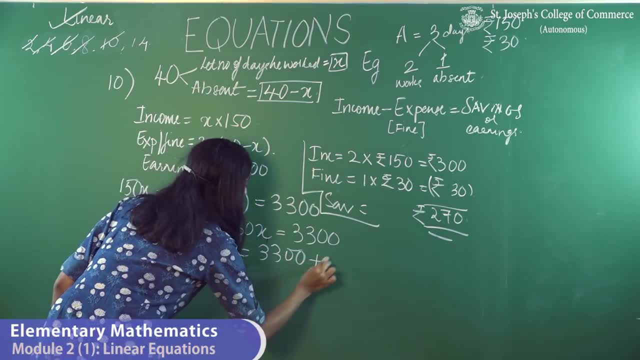 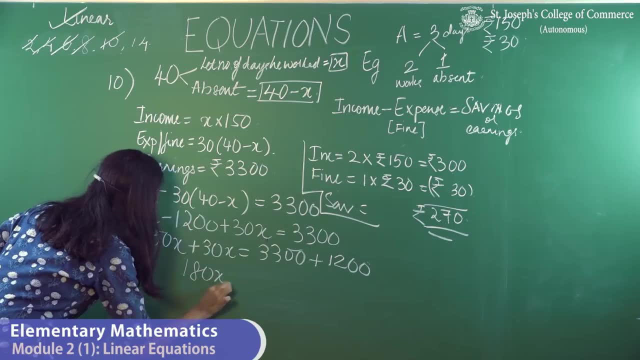 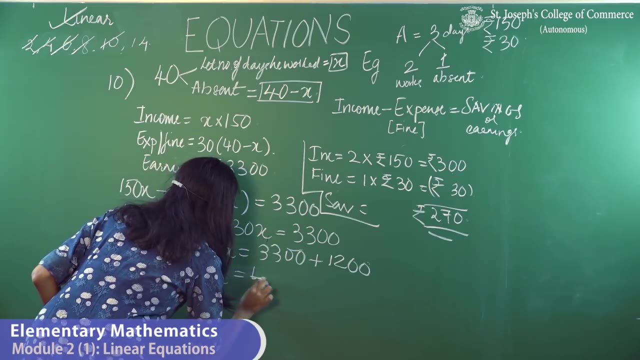 Rs.3300 plus 30x plus 1200.. When you solve it, you get 180x on this side, because 150 plus 30 is equal to 180.. 3300 plus 1200 is 4500.. When I divide 4500 by 180,, 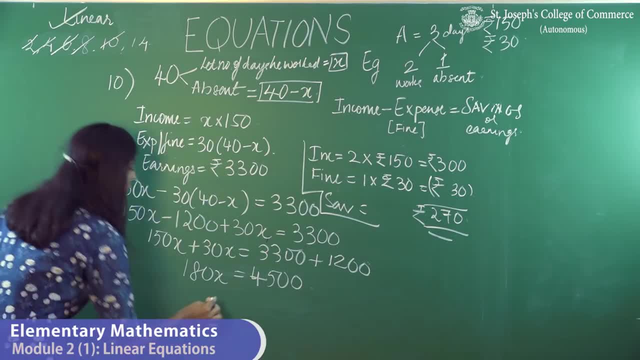 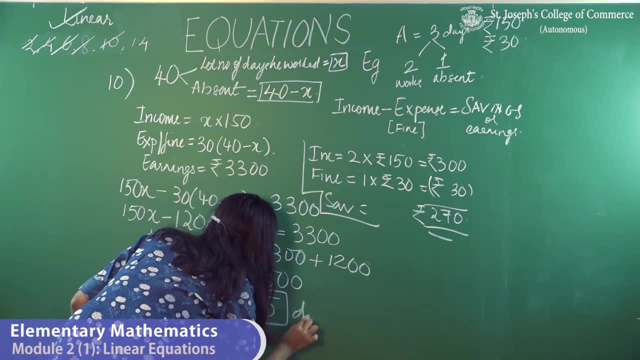 I get the number of days he has worked for. Therefore, x is equal to 25 days. Don't forget when you are writing your answer. the answer has to be: therefore, the person has worked for 25 days. This is the end of the question. 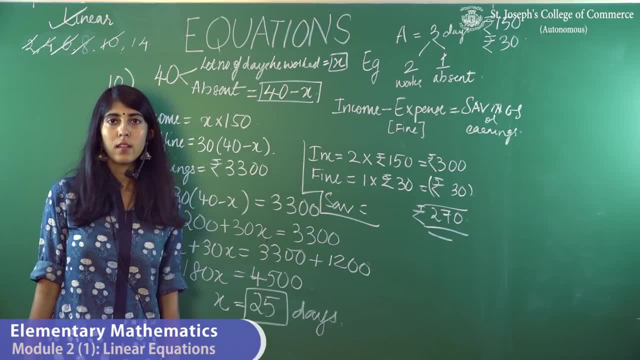 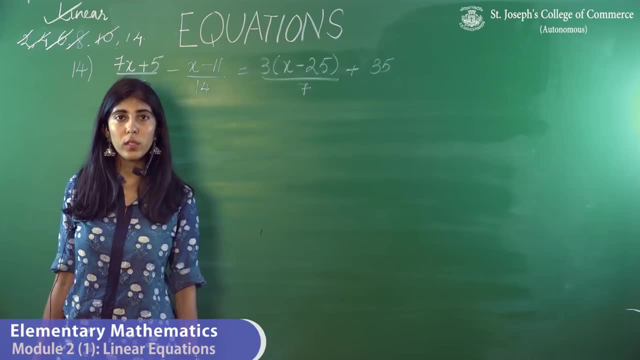 The next sum we are going to be doing is the 14th sum. This is the last sum under linear equations. This is the question. Again, if you notice, the question has a numerator and a denominator. Hence we must do the normal procedure. 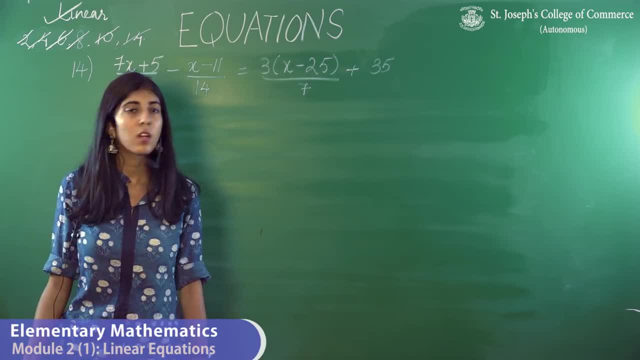 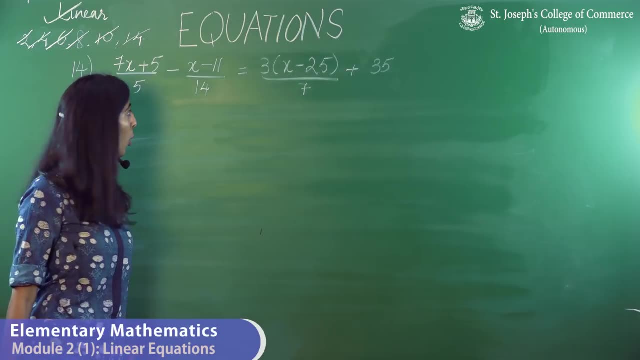 by following the equation. So this is the question. Again, if you notice, the question has a numerator and a denominator. Hence we must do the normal procedure by following LCM method, LCM of 5,, 14 and 7.. 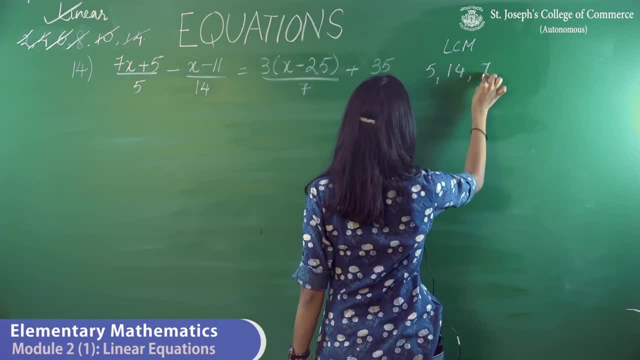 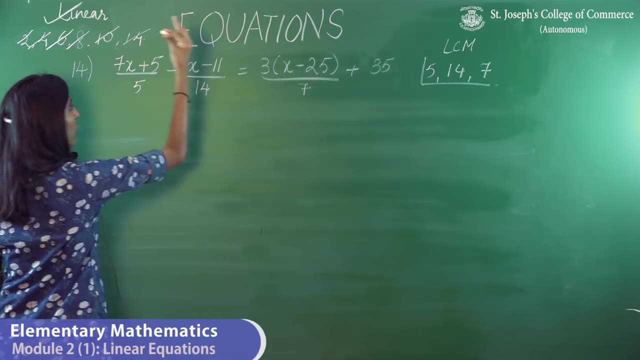 The reason I am taking all the 3 is because the basic concept is by shifting all the variables to the left hand side and leaving the 35 as it is, since it is a constant. So the first step technically will be 7x plus 5. 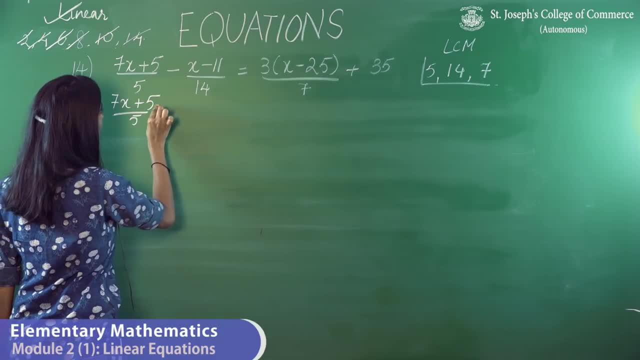 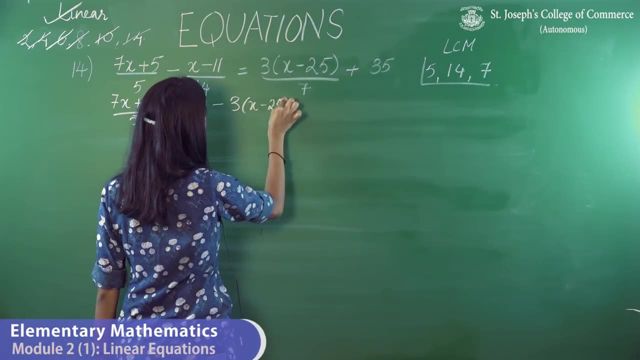 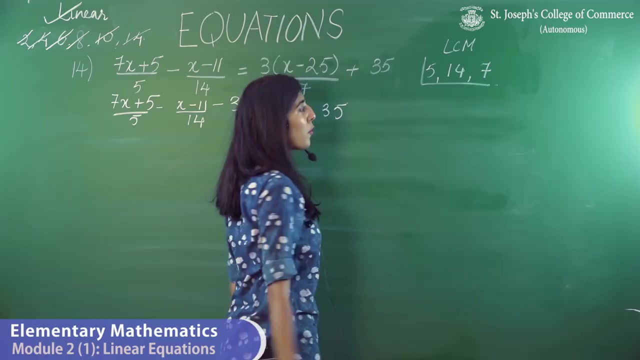 divided by 5 minus x minus 11, divided by 14 minus 35 plus 5 minus 3, into x minus 25, divided by 7, is equal to 35. This is precisely why I have taken the LCM of 5,. 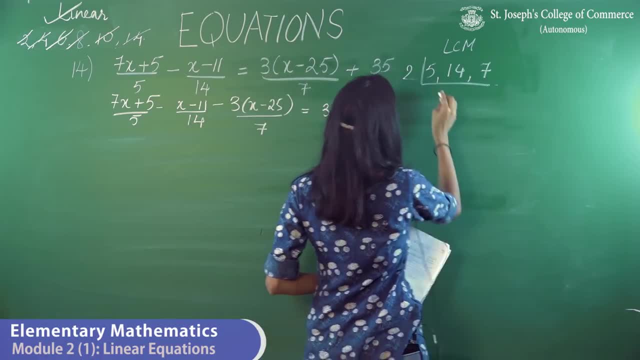 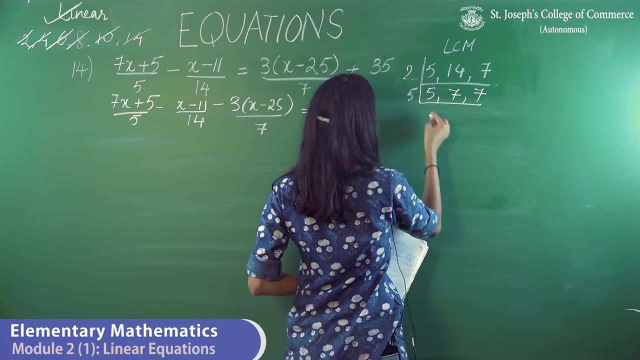 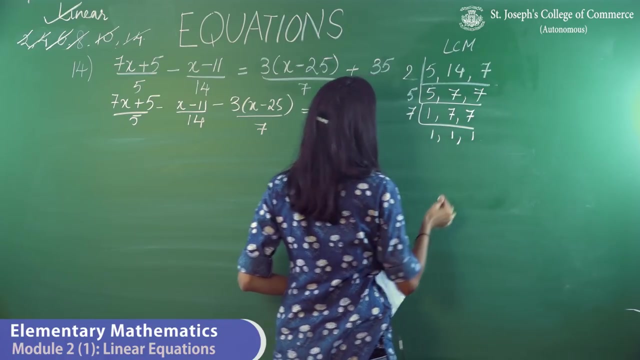 14 and 7.. So when I solve it, I start with 2.. Next I go with 5., Then I stop with 7.. This is the LCM of 7.. The LCM will be 2. 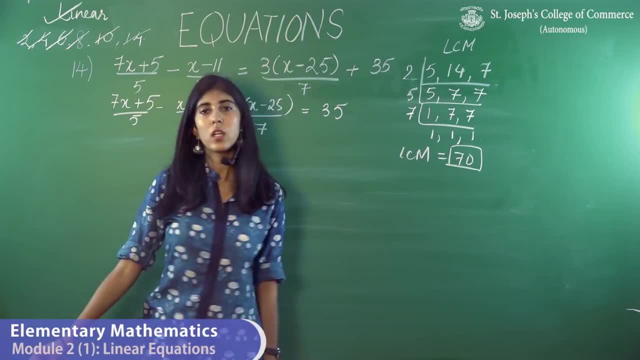 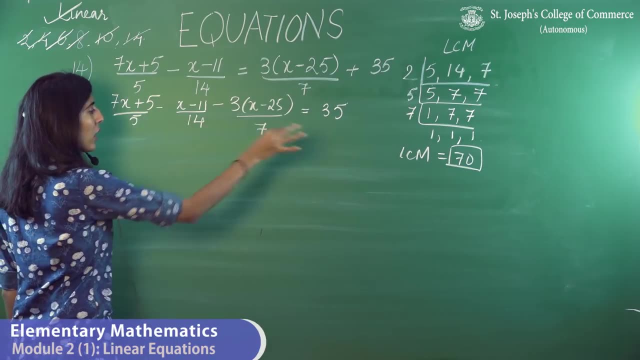 x 5 x 7, which is equal to 70.. Now that you have found out the LCM of all the 3 numbers, next you need to multiply the numerators with the same numbers in order to get the 70. So 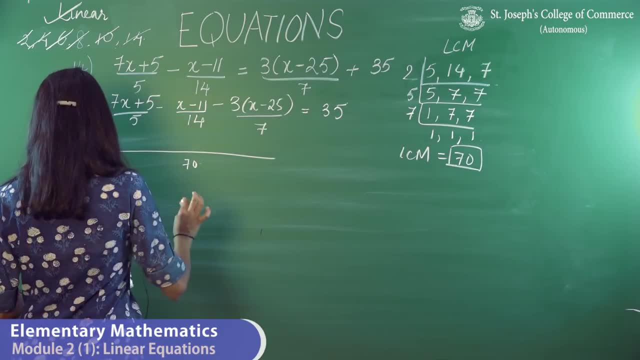 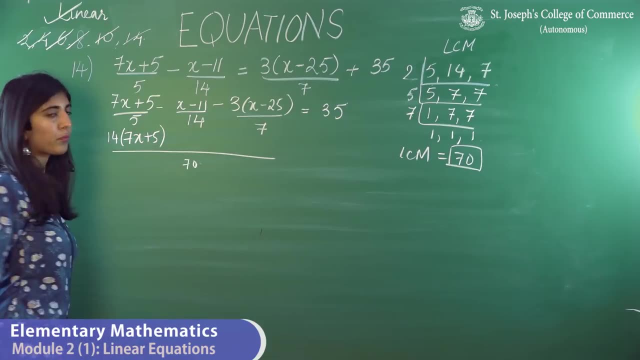 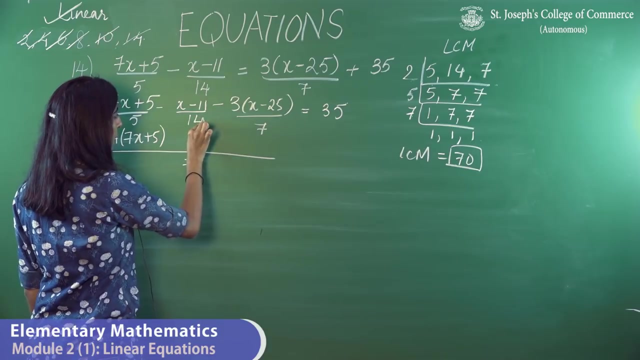 I start off directly by writing a 70 on the denominator 5, into what gives you a 70? 14, into what gives you a 70? 14 into 5.. So I multiply this by 5 and this by 5.. 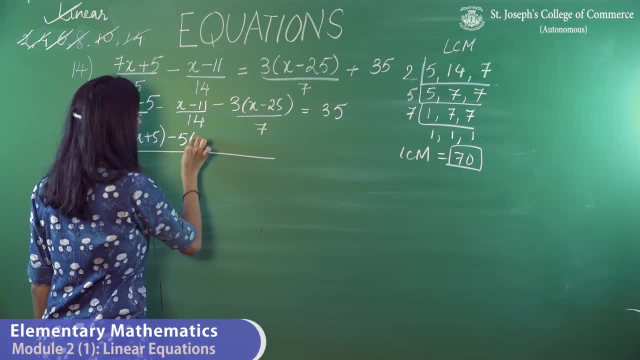 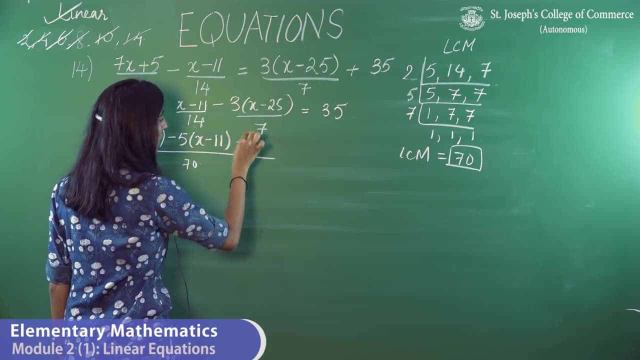 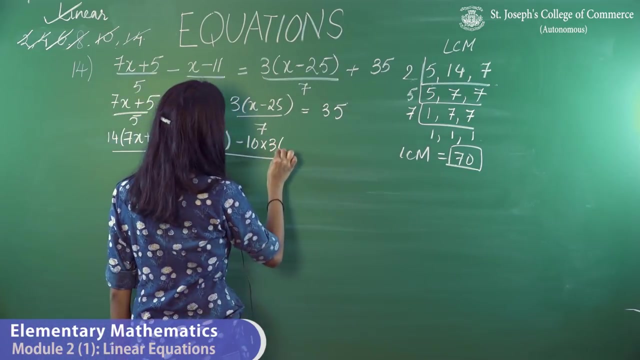 Do not forget the minus sign. So you do minus 5 x minus 11.. 7 into what gives you a 70? 10. So I do 10 into 3.. That means the number 3 into x minus. 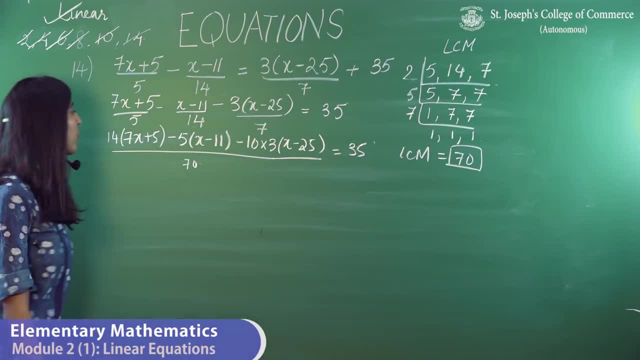 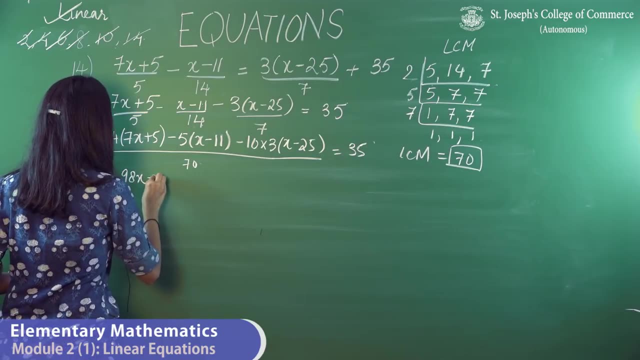 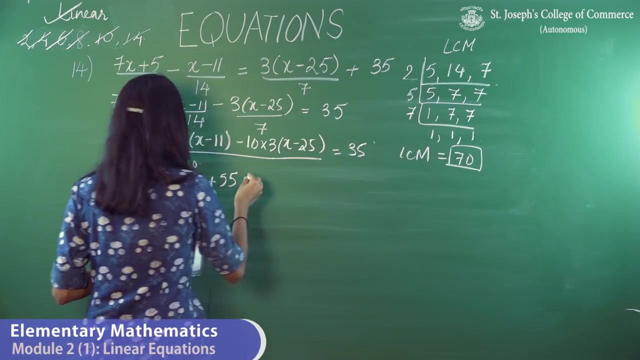 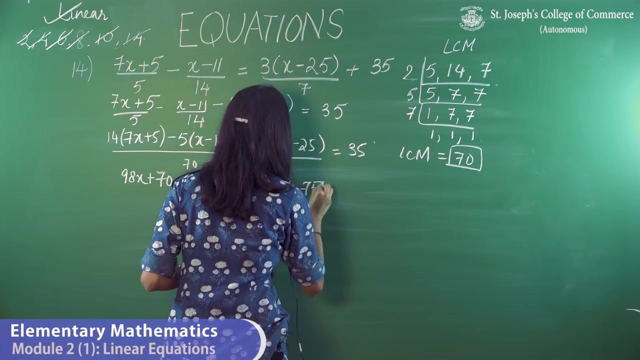 25 is equal to 35.. Moving on to the next step, I expand all the brackets 98 x plus 70 minus 5 x plus 55 minus 30 x minus into minus plus 750. whole divided by 70 is equal. 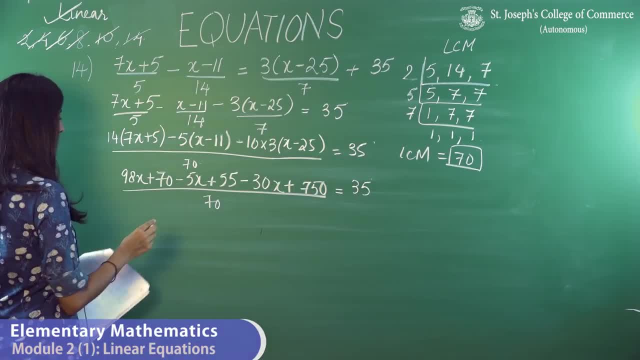 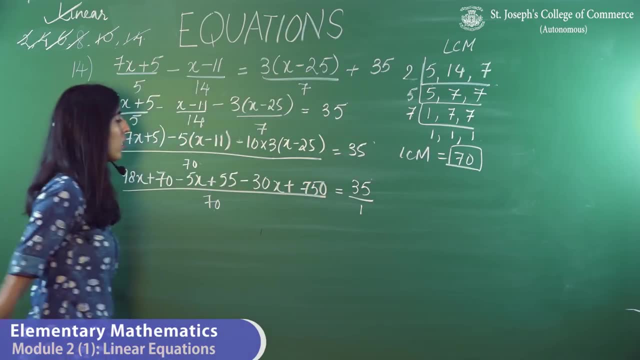 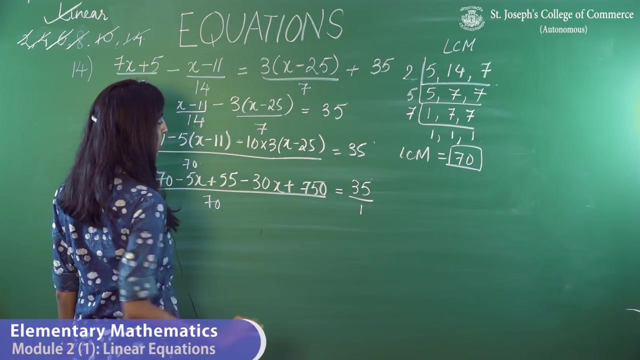 to 35.. The smart thing to do right now would be to take the 70 on the other side, because 35 does not have a denominator. It is technically 1.. So when I take on the other side, that means the left-hand. 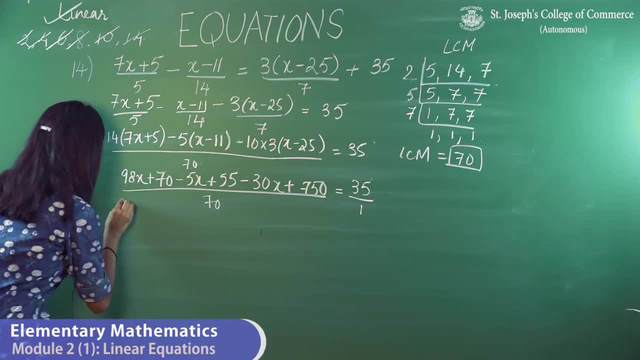 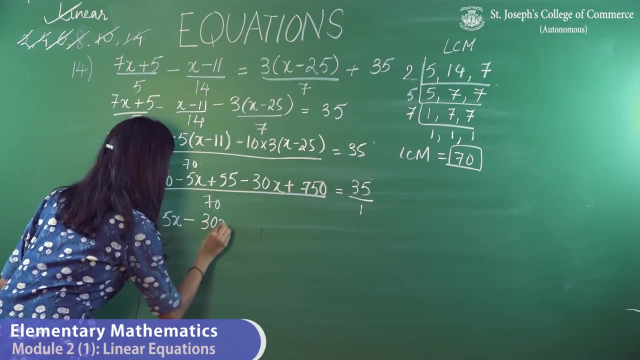 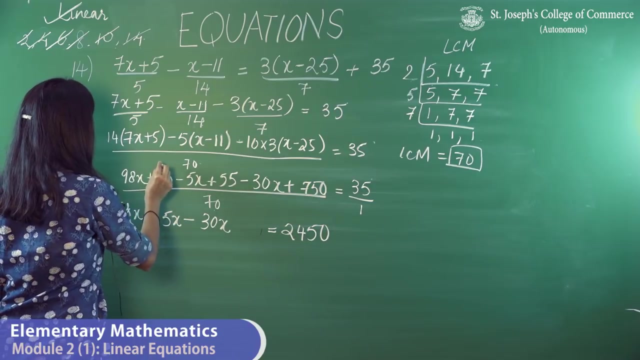 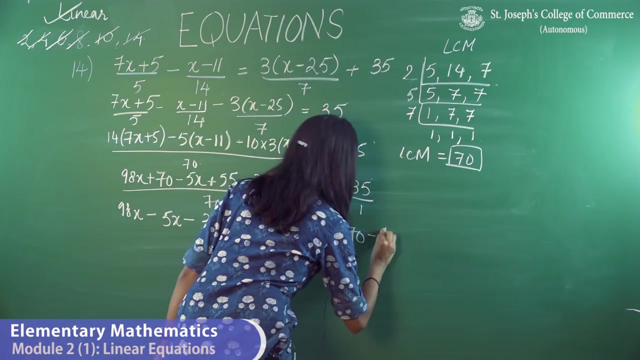 side will have so many variables and the right-hand side will have only 35 into the left-hand side. So I would take all the constants from here to the other side. Plus 70 will become minus 70.. Plus 55 will become.